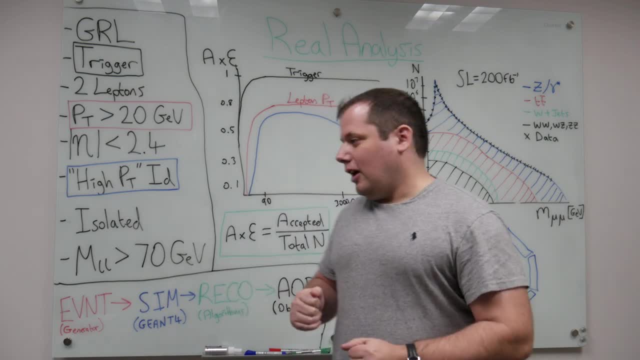 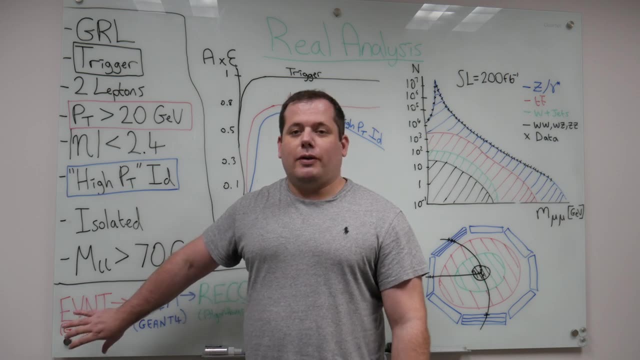 of course, the real data is going to give us the answers of whether new physics exists or not. What we have to do with the simulation is we start with the generator to generate all of the different standard model processes and even beyond the standard model processes. 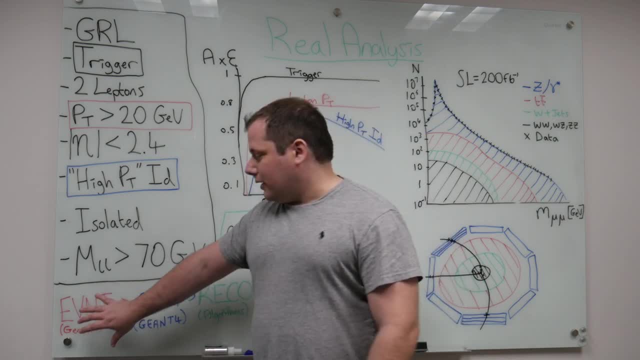 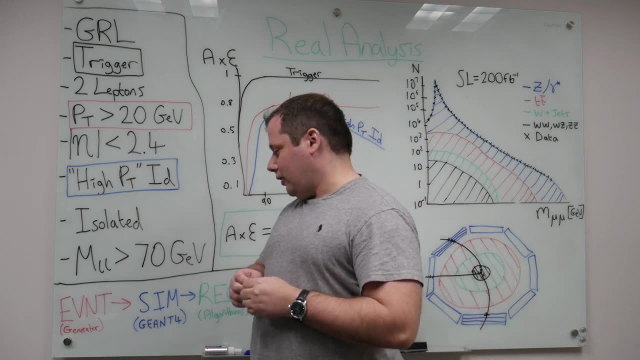 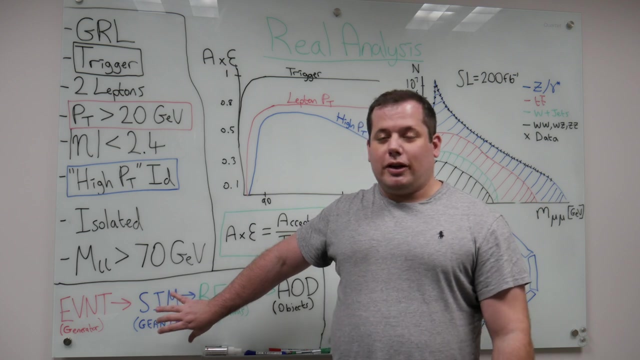 that we know about, Then what we have to do- because that's just generating the PP collisions, creating the particle and then its decay products- what we then have to do to actually see what the detector would see- is we go to the next step in the chain called simulation. 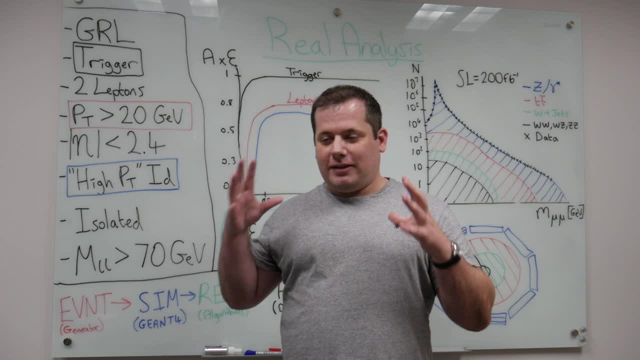 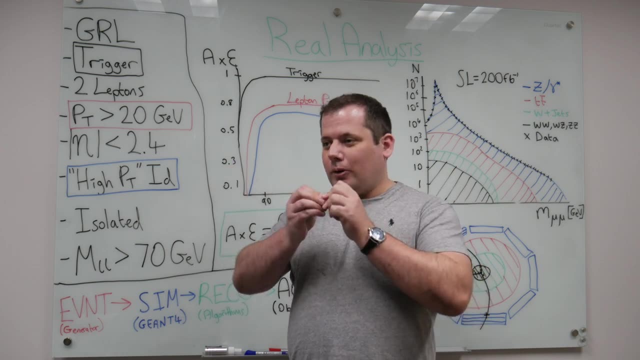 which essentially wraps the real detector. We have to do the same thing with the detector. We have to do the same thing with the detector- or our best description of the detector- around that underlying event. It also simulates not just the single proton-proton collision but all of the pileup of other collisions that. 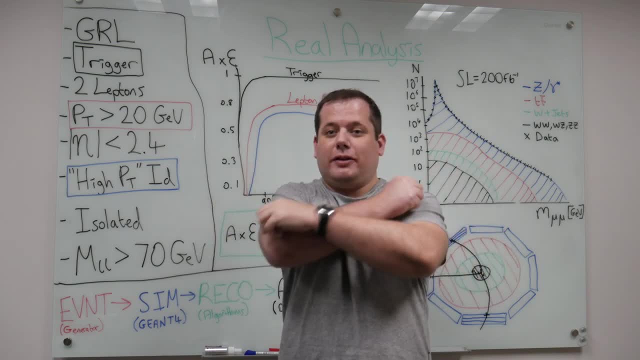 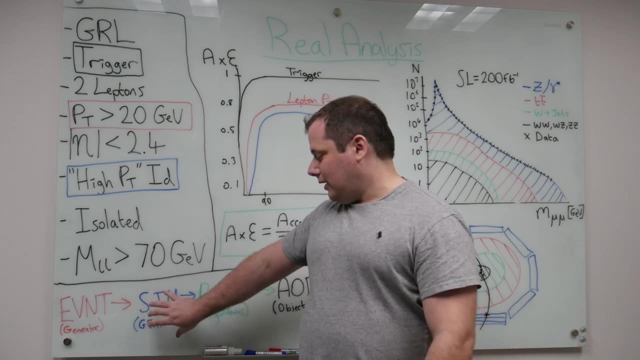 may happen because we have bunches of 10 to the 10 protons passing by each other every 25 nanoseconds. So any of those secondary collisions are also simulated at this point. The program that does all of this extra simulation of the detector is called Géant4.. It's actually 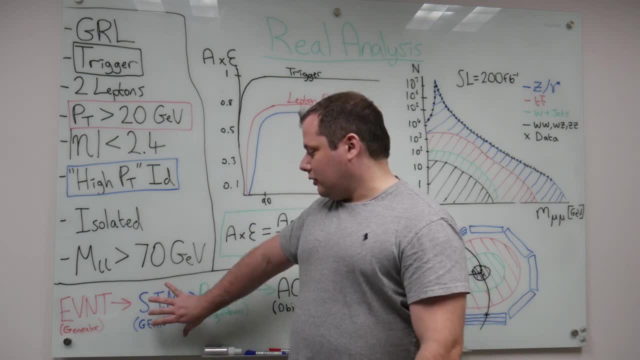 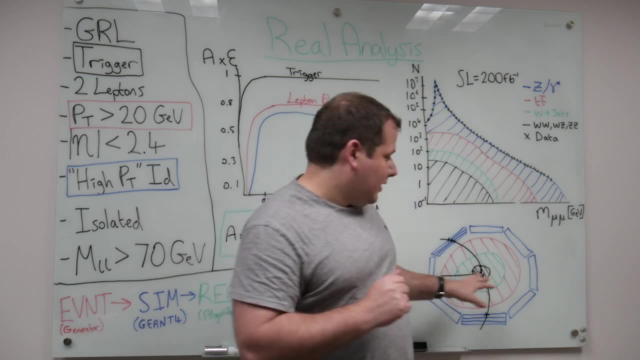 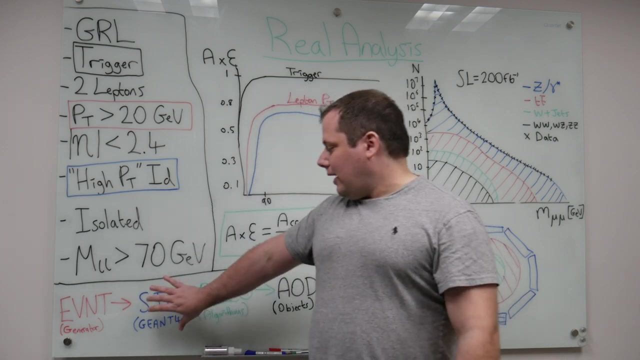 used in many particle physics programs. And then once we've kind of seen how the detector reacts to all of these particles traveling through different parts of the detector, kind of like I drew earlier, and it would leave ionization tracks and energy deposits and so forth- the next step is then to run. 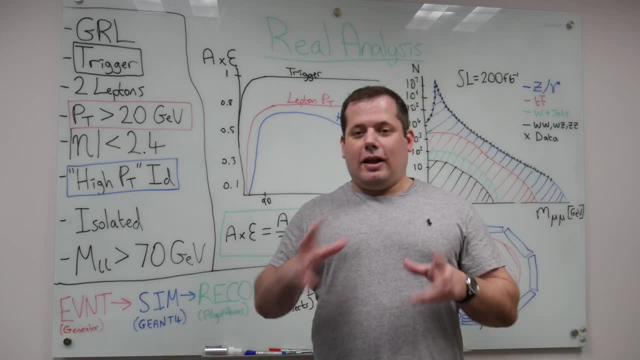 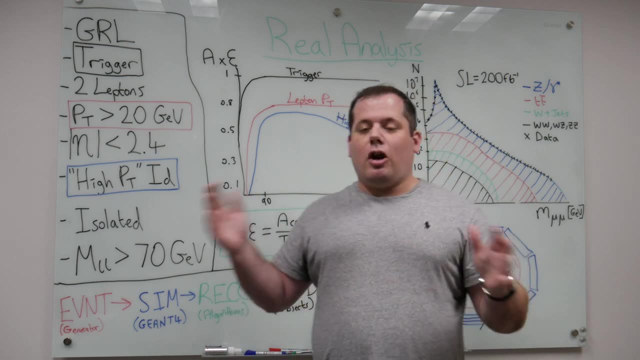 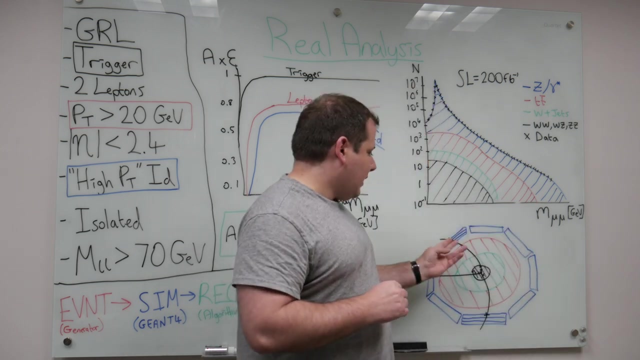 all of our reconstruction algorithms over all of these hits and deposits in the detector, to try and understand what they mean. So here, the big coding framework that is used is called Athena, but basically it's a number of different algorithms, So that let's say, you know we. 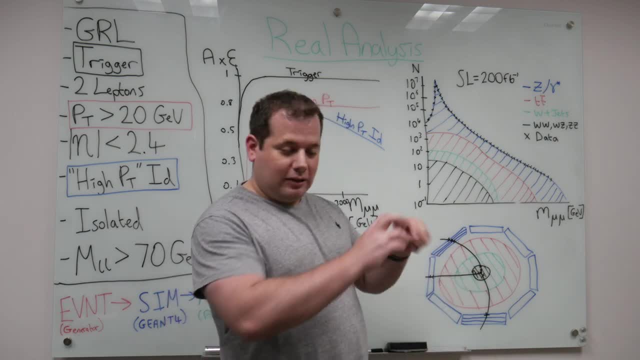 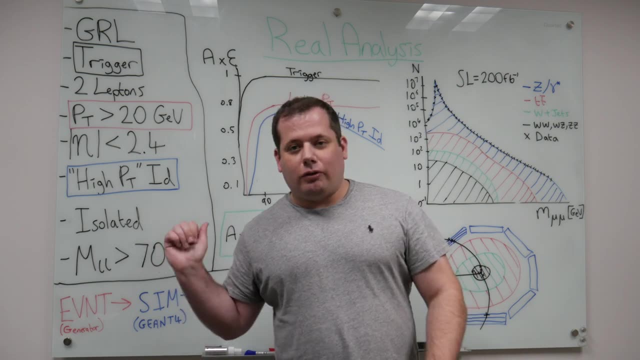 were looking for muons and we had tracks in the inner. we had deposits, ionization deposits, in the inner detector and we also had some hits in the muon spectrometer. Well, what the reconstruction algorithm would do would try and turn those hits into a muon. So we 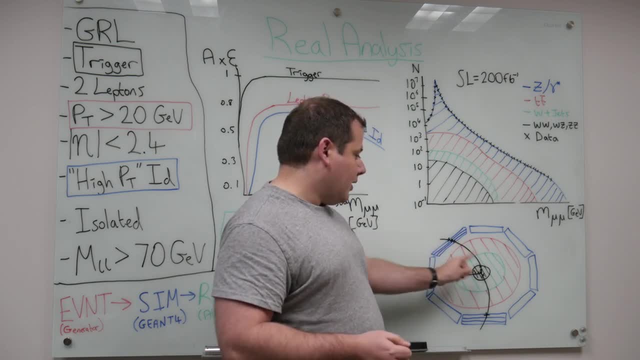 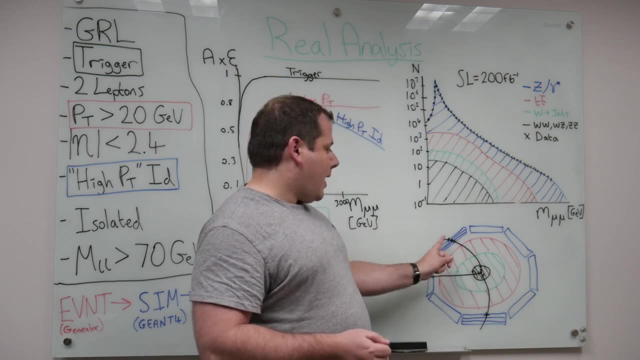 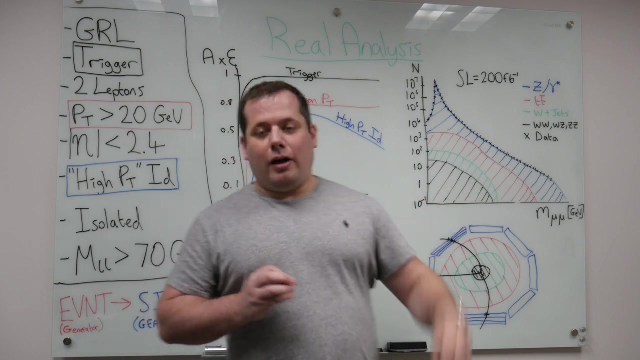 try a number of fits to try and fit a track through all of these hits inside the silicon in the inner detector and the TRTs in the inner detector and so on and so forth. So that's what we're trying to do. So the reconstruction stage really tries to turn all of the signals that we get from the 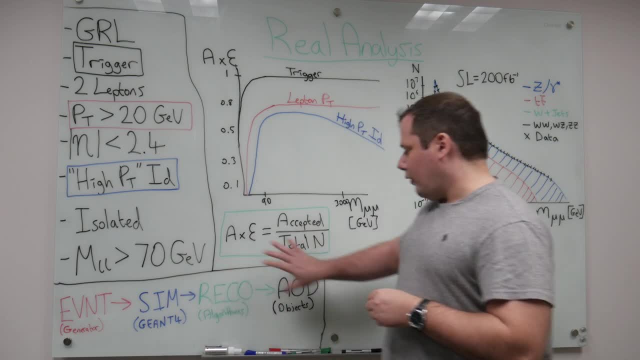 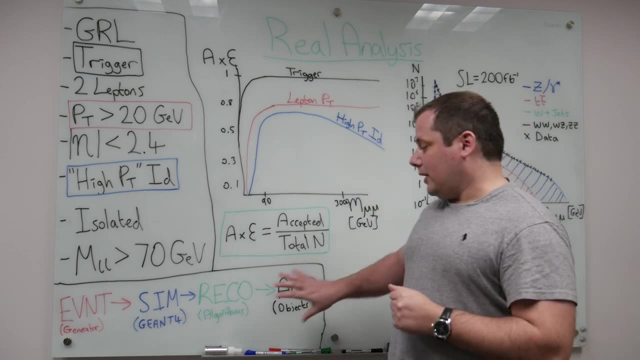 detector into recognizable objects. And then, finally, we have this AOD stage, where all of that information gets simplified and put in the object-oriented format that we can then as experimentalists, use. Okay, So this is the full change of the muon spectrometer. 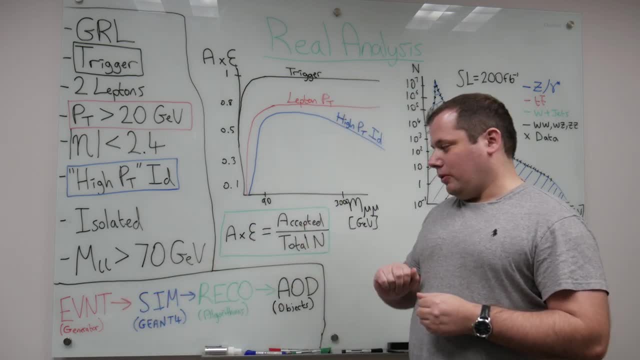 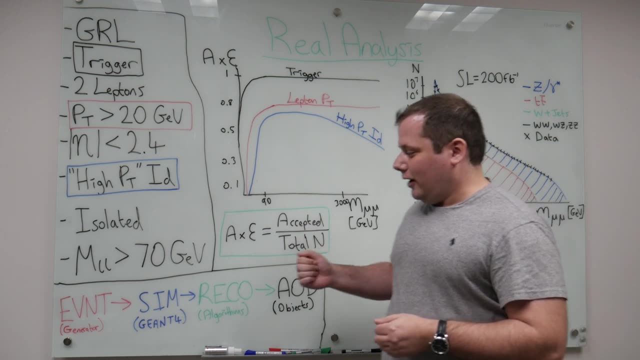 So the muon spectrometer is the same when we're doing the simulation of every physics process that we're interested to look at, whether it be standard model or beyond the standard model. physics- And really data- takes a shortcut here. right Nature provides us. 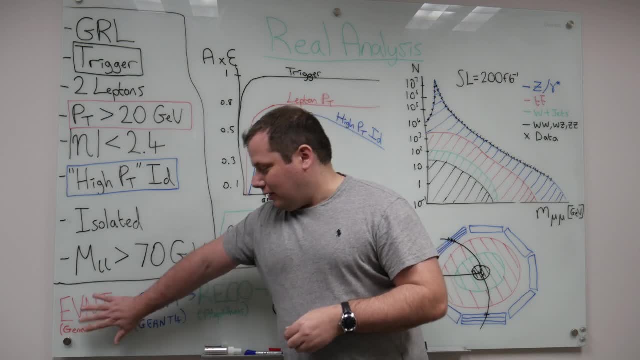 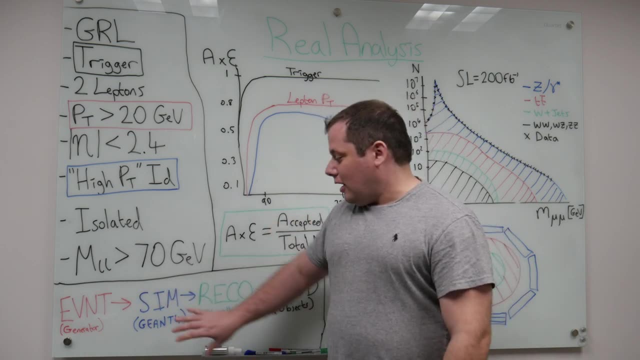 with the LHC colliding protons, provides us with this information in real data which we can't really see right. We can't look at the truth, information in data. The real detector gives us this part right for real data. We have the electronic signals which 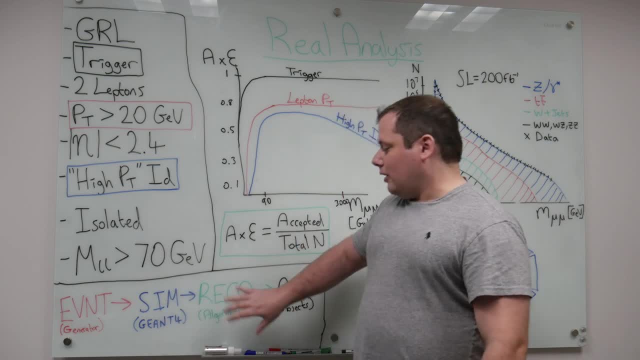 are being read out from the real data. We have the electronic signals which are being read out from the real data. We have the electronic signals which are being read out from the real part of the detector. And then where we connect back in with our simulation is that we run. 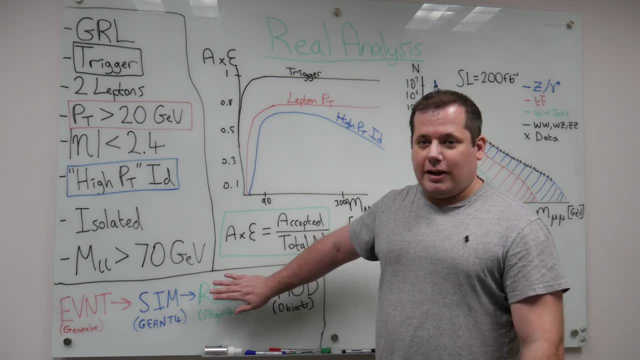 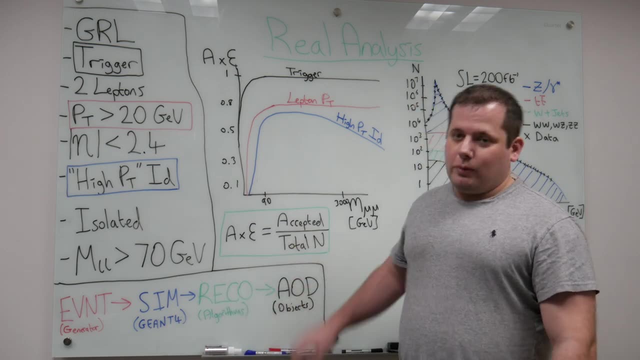 the same reconstruction algorithms that we run on the simulation, We run that on the real data as well, And then we do the same conversion of the real data into our final AOD objects. So at that stage we can analyze real data and we can analyze our simulations. 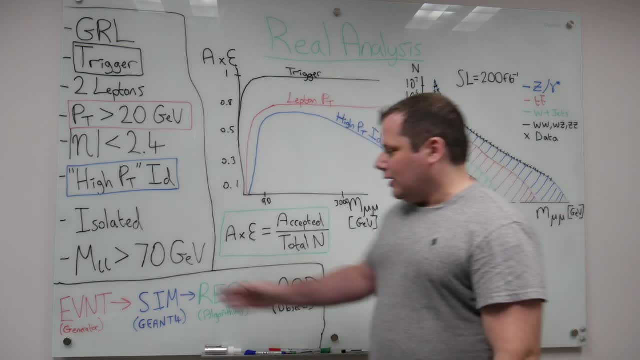 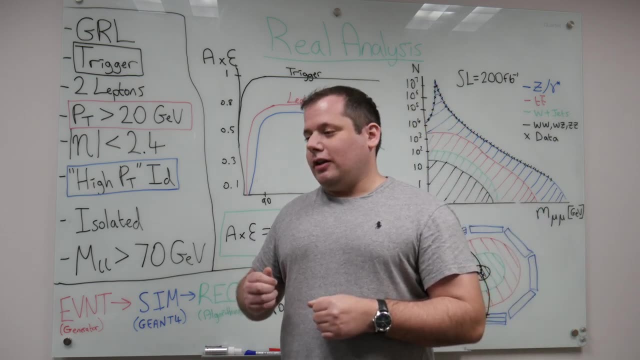 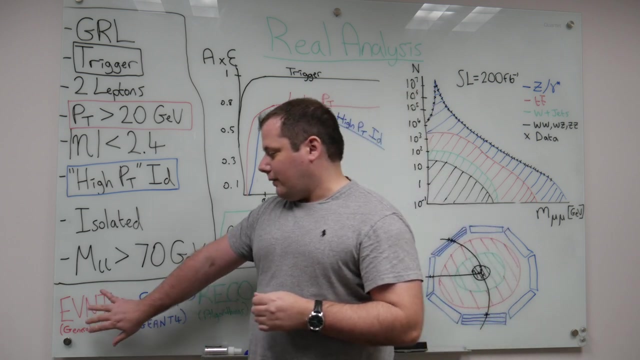 and make a one-to-one comparison between them. Now, when you were doing the selection and looking at the different variables from the Z' prime events previously, you were looking at some simple variables like the transverse momentum and the eta and phi direction. Okay, so those are things that you have accessible. 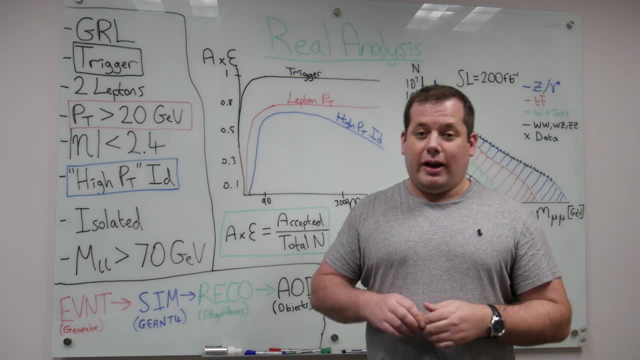 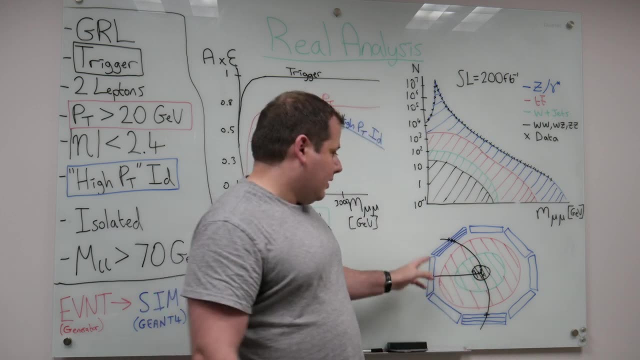 here. but as you build up this real picture of an event and the objects in it, things get much more messy, right? So you could have, for example, in the real detector, you could have tracks which don't fit well, right. Maybe not all of these chambers had hits in them. 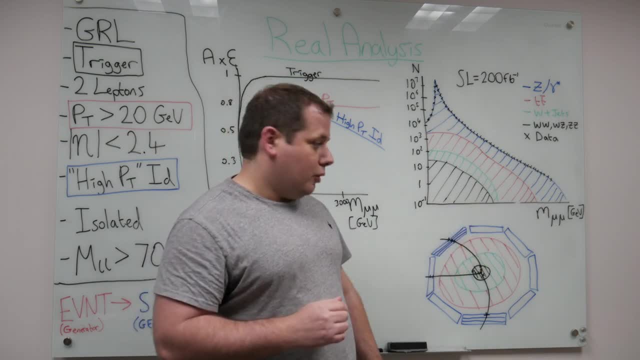 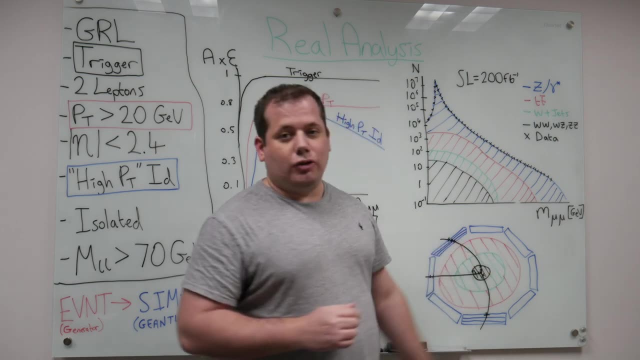 so you couldn't get a very good fit going into them. So that's something that you can fit going through to give you your muon. Or maybe you had an electron that was so energetic it punched out of the electromagnetic calorimeter and into the hadronic calorimeter. So how do you know? 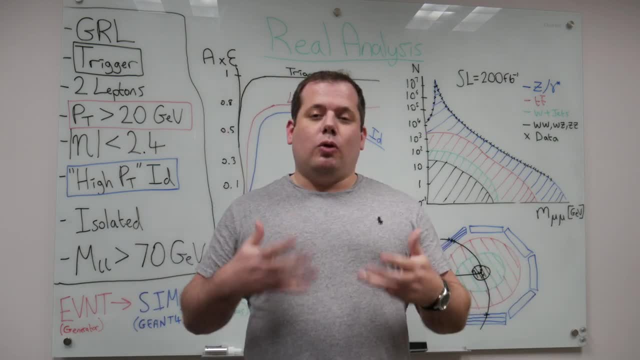 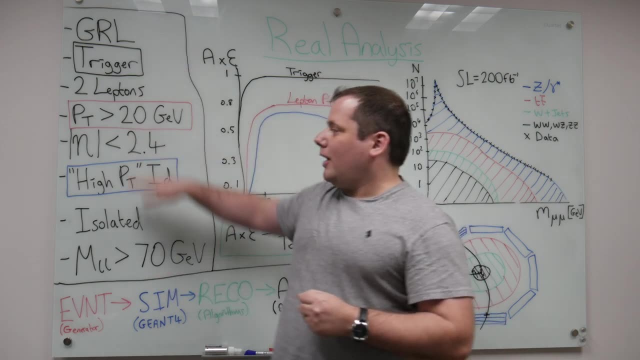 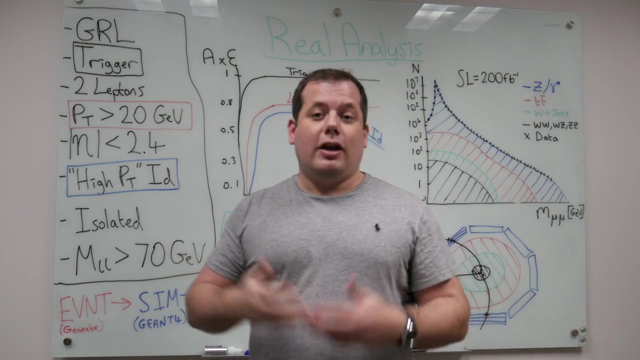 whether it's a jet or it's an electron, And these are real world decisions that we have to make as experimentalists. So, if I take on the right hand side here, this is an event selection that would be applied in a real analysis, looking for, let's say, a z-prime decaying to two muons. Now, let's. 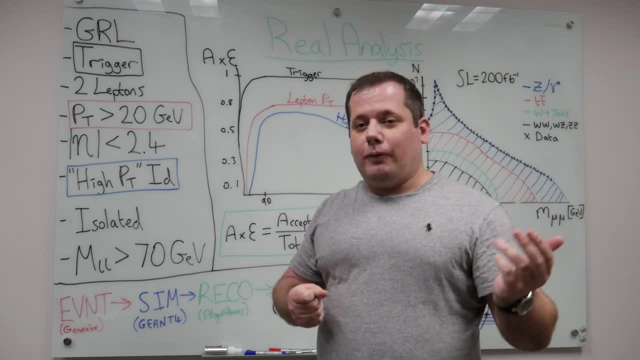 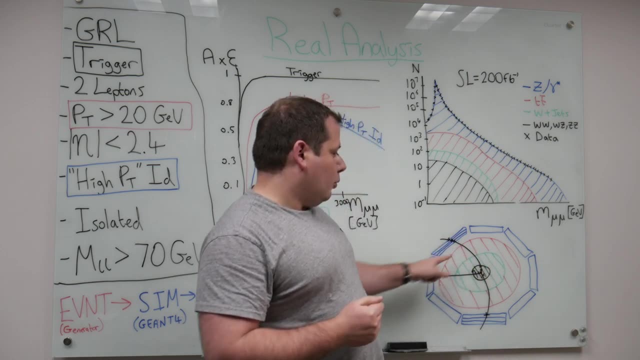 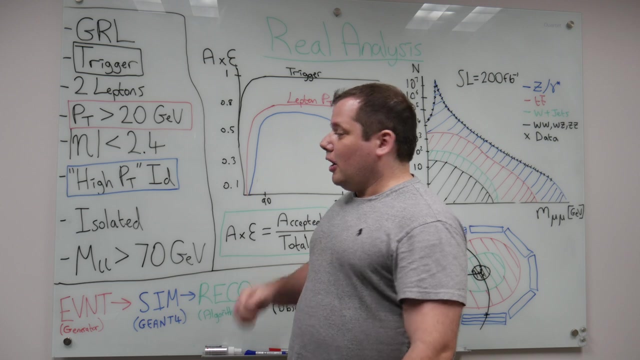 take muons just to move over. We were talking about electrons before, still leptons, but here, instead of looking for deposits in a detector, we'll be looking for objects that traverse all the way out to the muon spectrometer. But the analysis for two electrons would be very similar. So what we would? 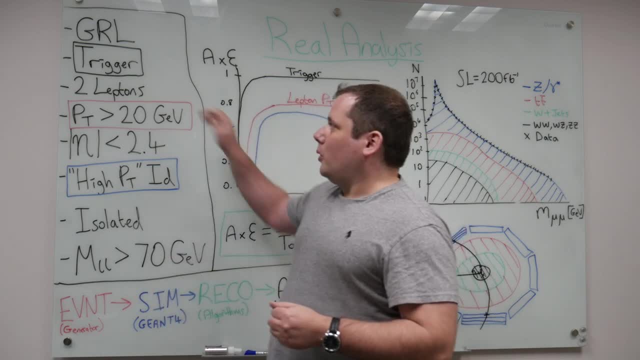 ask when we're doing our real analysis. so, first of all, when you're looking at data, you have something called the gamma. So what we would ask when we're doing our real analysis. so, first of all, when you're looking at data, you have something called the gamma. So what we would ask when we're doing our real analysis. 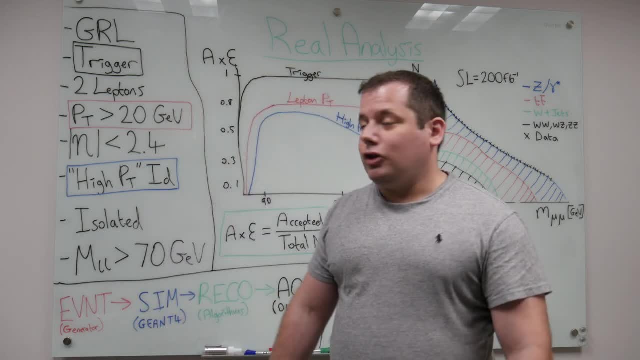 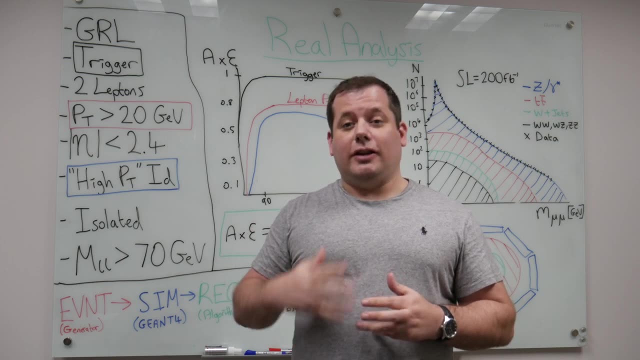 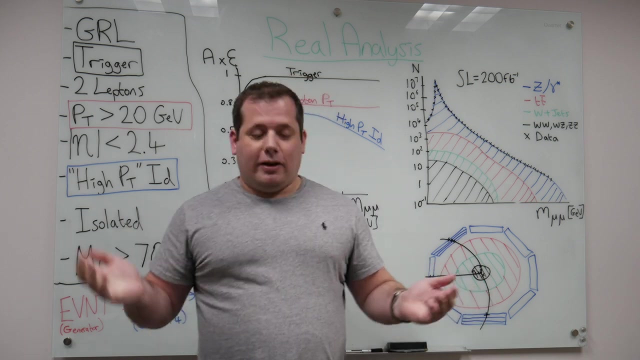 good runs list, the GRL. so I won't go into that in too much detail now. But basically it's a set of flags that tell you if the detector was operating nominally during the time that we were taking the real data. You know, let's say that in a detector the power went out or maybe there was an extra amount of electronic. 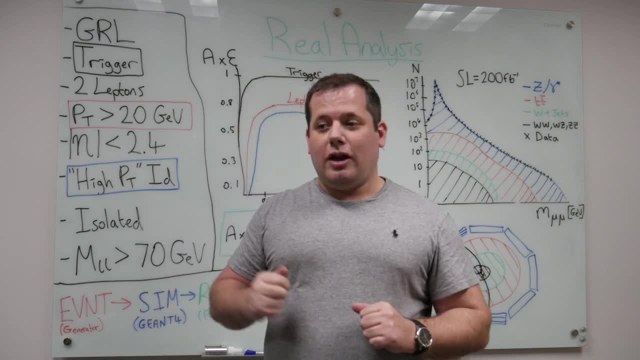 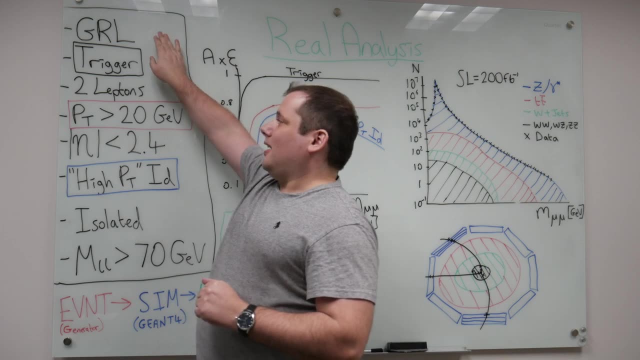 noise in the ecal so you can't get good readings for electrons. Then a flag will be switched that says don't use real data during this period. So this one actually only applies to data. but it would then allow you to make sure that. 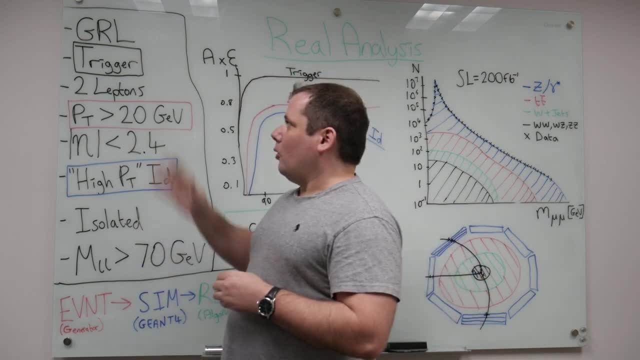 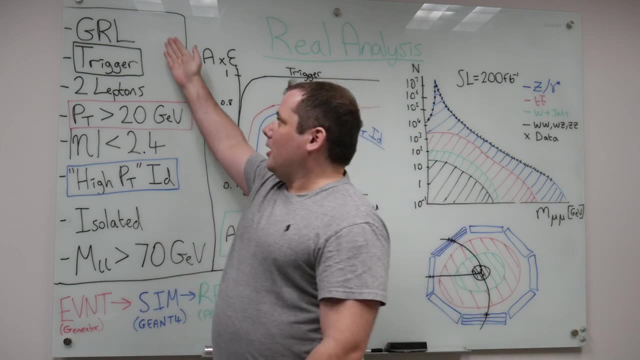 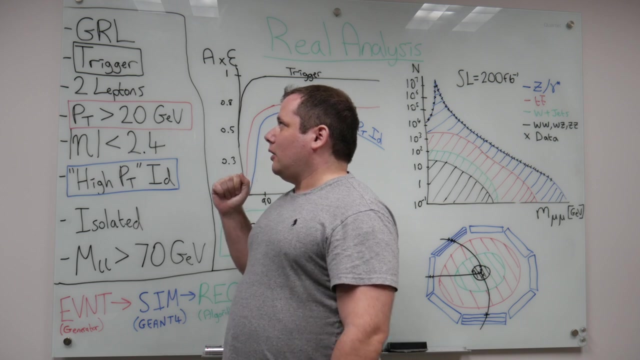 the data you're looking at is of the highest quality, So automatically everything in the simulation passes that, because we simulate ideal conditions and we make sure that matches the data by making sure that data also then passes these threshold conditions. So then we go on to the next cut that you would make. 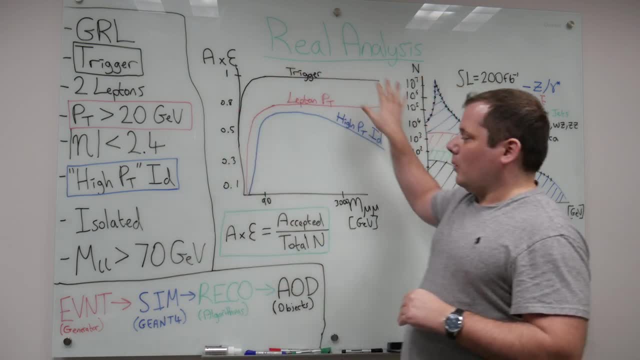 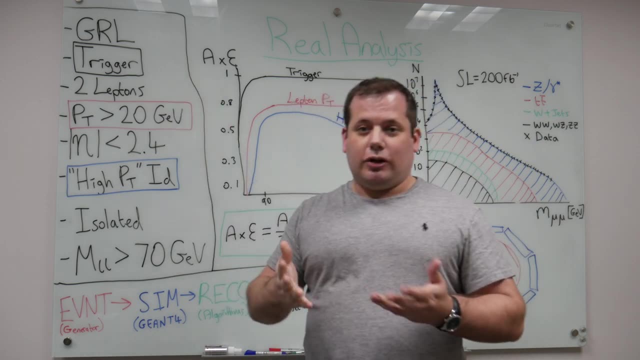 So in each of these cases, you're going to come to this diagram as well as the amount of events you're accepting into your selection. Let's take the trigger, for example. So I talked earlier about the fact that we have over 40 million collisions per second. 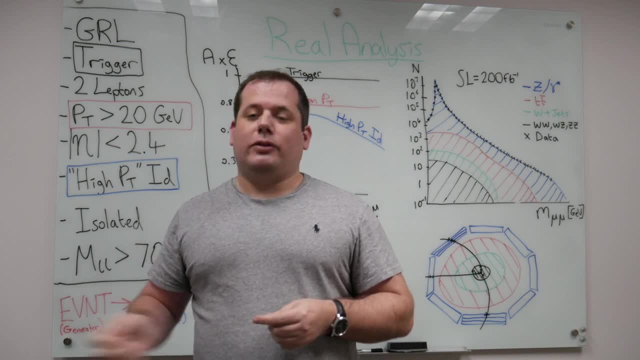 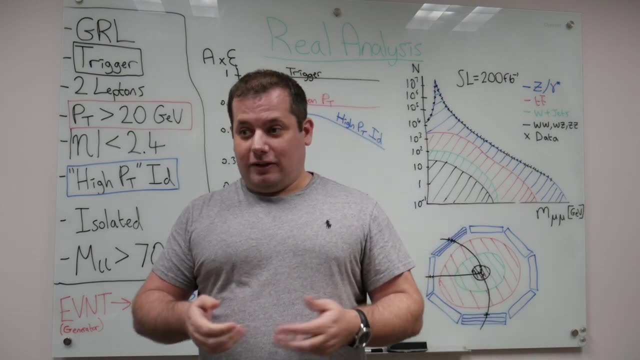 at the LHC and we're only able to write 1,000 of those per second to disk. So this is where the trigger menu comes in and there are many triggers that are run on the real data to then cut down how many events. 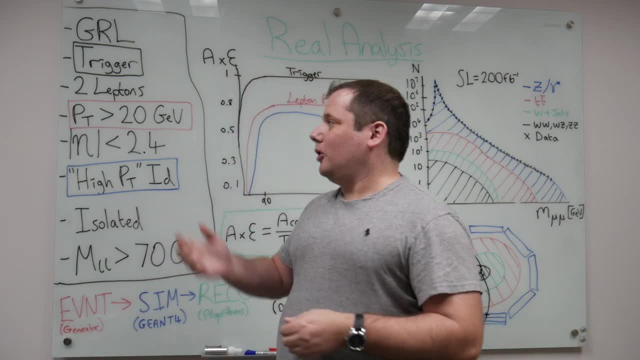 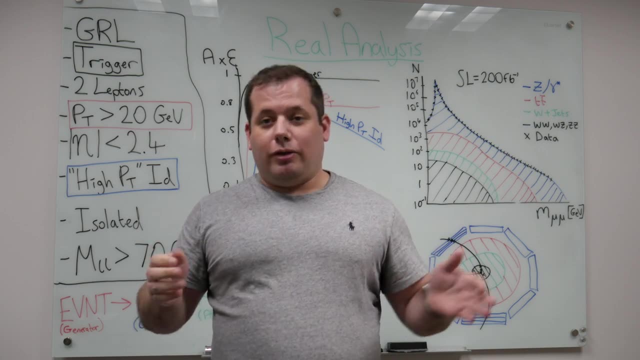 that you will actually see, And so, therefore, in our simulation, we also have to recreate that fraction of events that we would collect out of the total that would be passing through the detector. So if, for example, let's give an example of a trigger for muons, 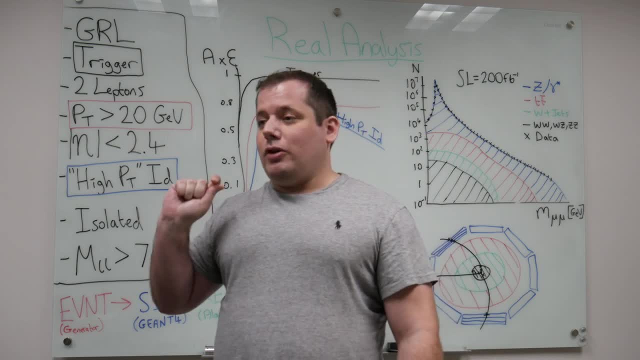 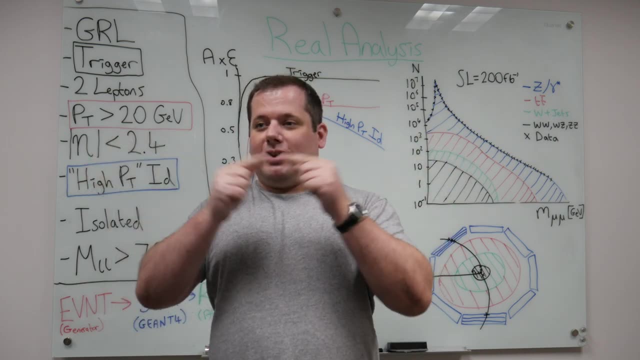 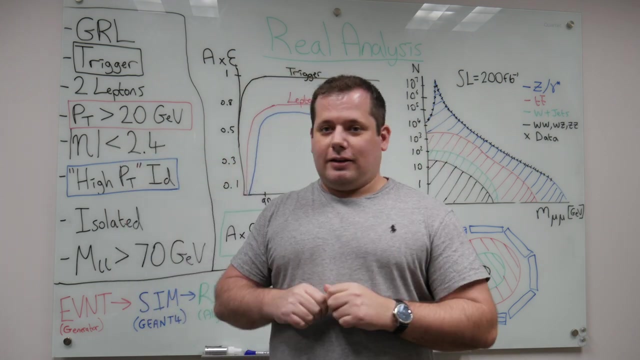 You might say: OK, record this event if you see two muons that have a PT of greater than 15 GeV. So every time it sees an event which has two muons Which have a very low but meaningful threshold of 15 GeV, then it writes that to disk. OK, 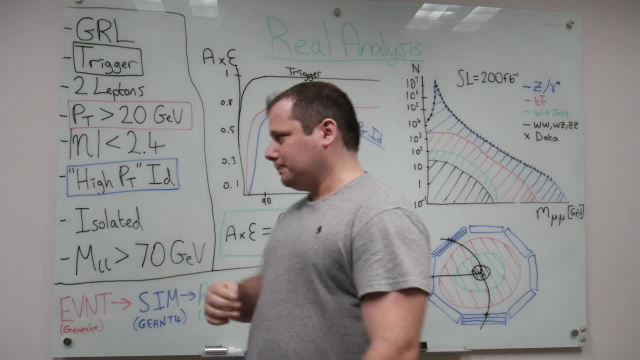 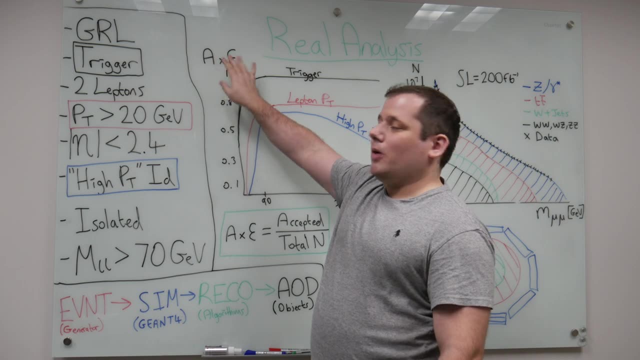 Now, we can't record all of those events. Some fraction of them get recorded, And so we'll come to this plot for the first time, which is the acceptance times. efficiency: Basically, how many events are you selecting out of the total possible versus the dimuon? 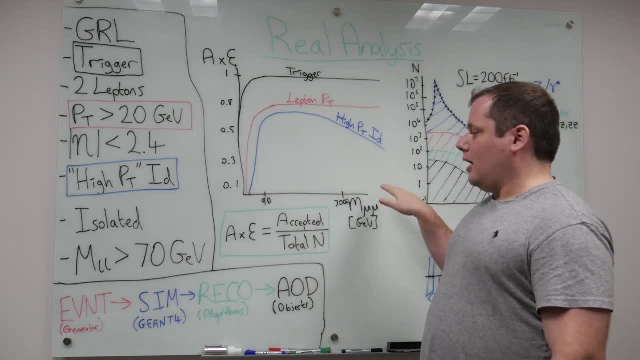 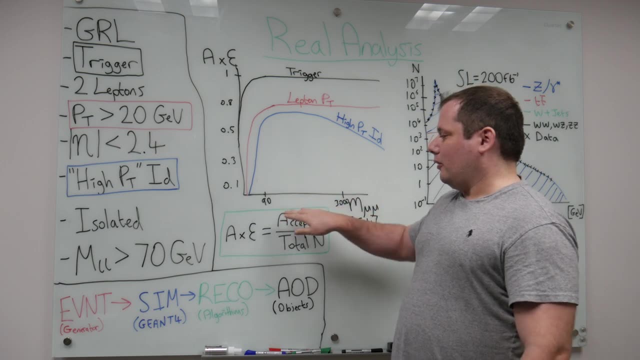 invariant mass, so the mass of the dimuon system. OK, And so the way you calculate this is. you know, at truth level, At least with the simulation you could figure out what the mass of your dimuon pair is. 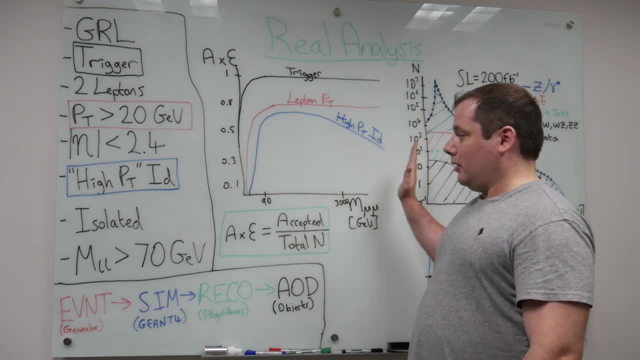 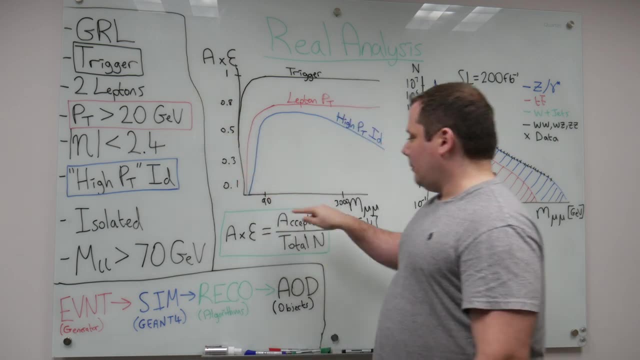 And so, for your total sample, you might say you have a certain number. Well, now let's see how many of those pass each of these selection criteria. So, for example, if we take the trigger, which is this first line, at very low mass, well, 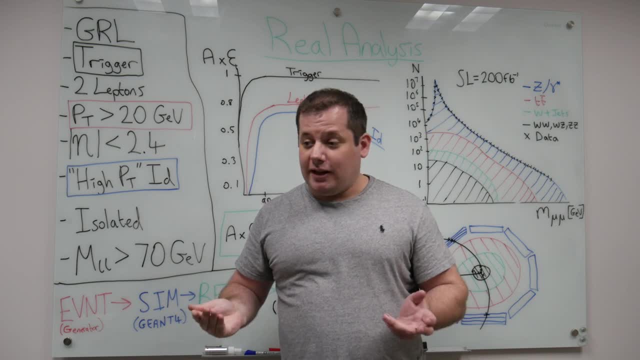 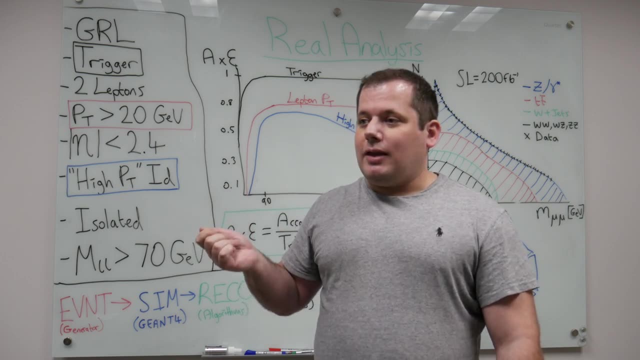 maybe the leptons are below 15 GeV PT. Therefore the trigger- let's say there was one muon with 10 GeV, With 20 GeV, OK, Therefore that wouldn't pass this trigger which is requiring two muons to have greater. 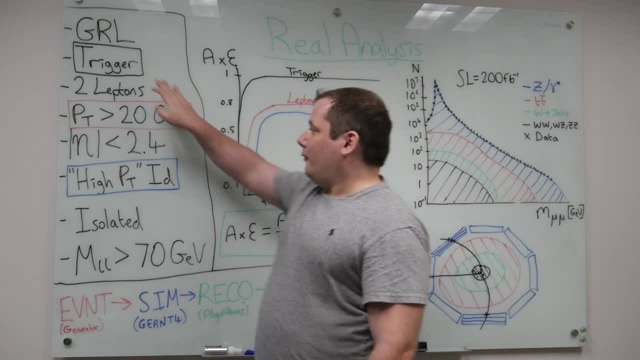 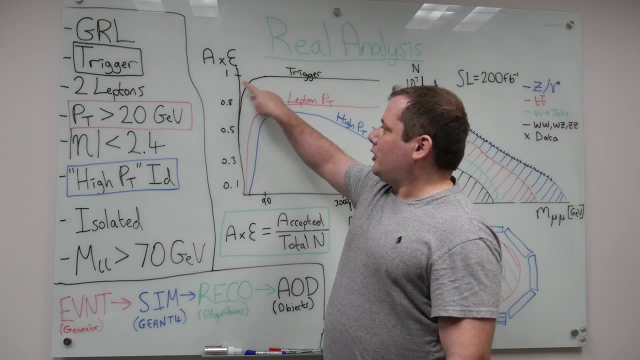 than 15 GeV. Therefore, if the trigger doesn't fire, then even though you had an event with this 10 and 20 GeV muon, it wouldn't select it right. So your efficiency is then less than 1, because the total number you're accepting is maybe. 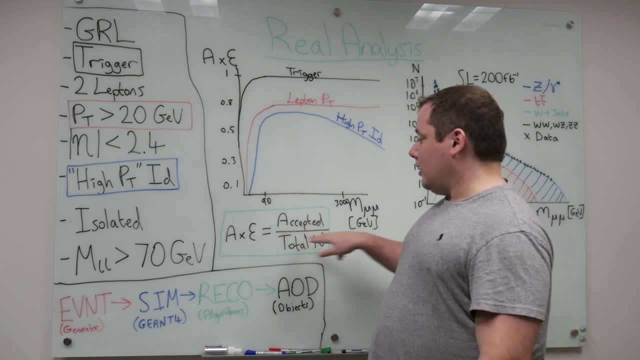 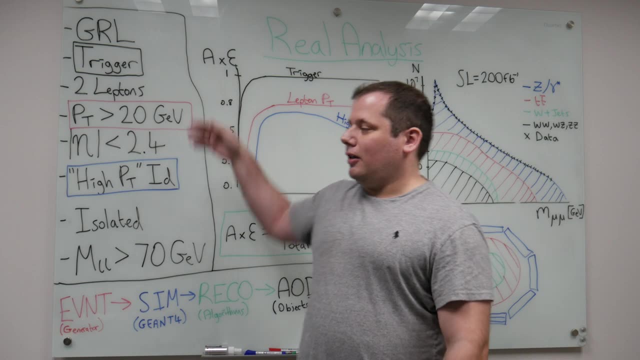 8, and out of the total number that were in that range was 10,. so you have, say, an 80% efficiency there. OK, So if you get to higher and higher mass, that's implying that the momentum of the muons is. 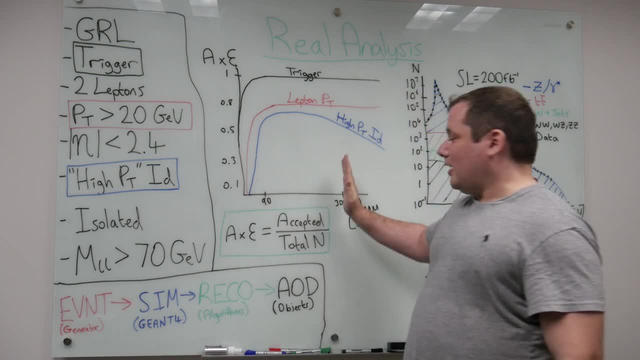 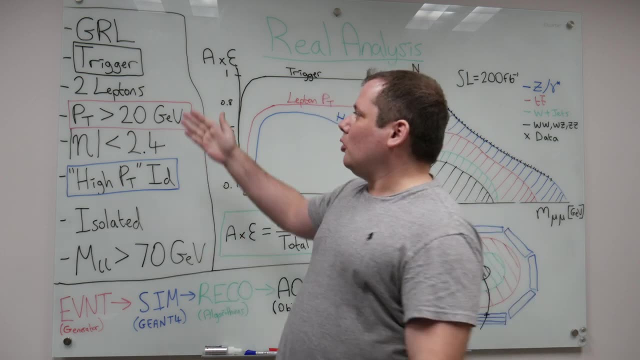 higher and higher. therefore, you know, if you're out at 3 TeV, then all of the muons are going to have a PT way higher than 15 GeV, and so you'll see almost all of the events, because they have way higher than two muons with 15 GeV. 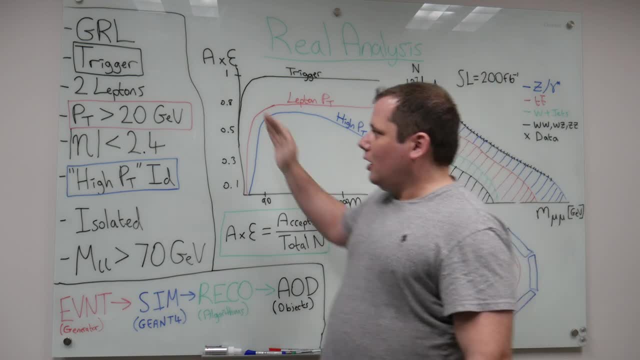 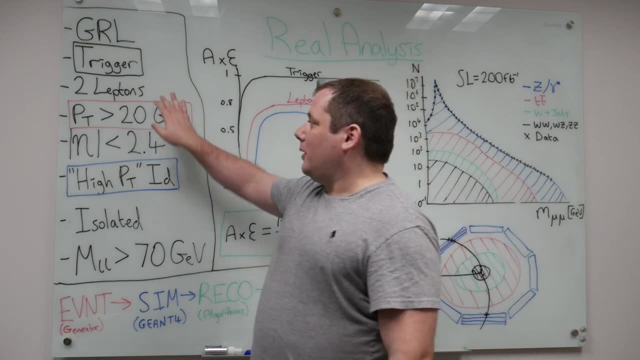 So the efficiency is very, very high out here. Then the next selection that you could make: well, we're interesting in Z prime decaying to two leptons, or two muons in this case. so we can just simply ask: are there two or? 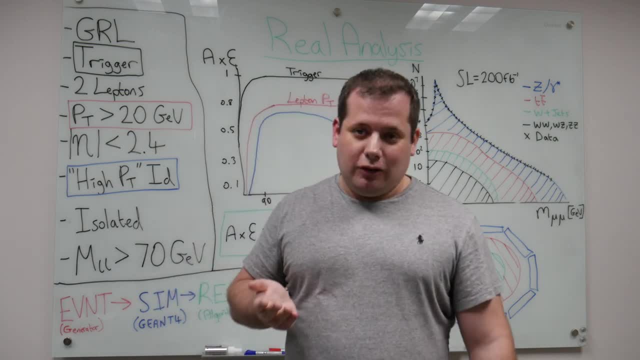 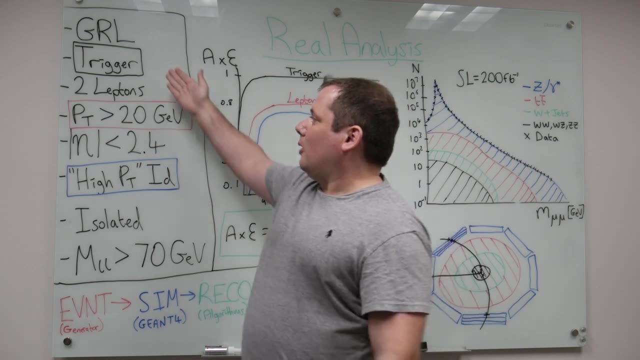 more muons in the event. Maybe you want to ask for exactly two muons. OK, So you'd have some efficiency loss because there'd be events with one muon in it. well, maybe not because of the trigger, but if you ask for exactly two, then there would be some. 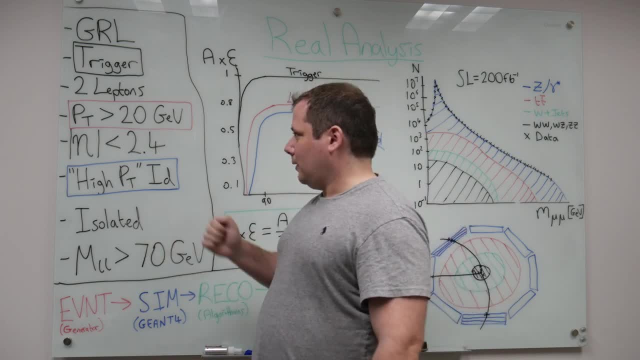 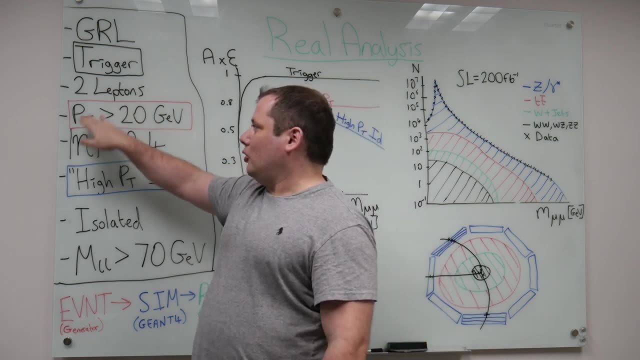 events with four muons in it and so forth, so you can cut those away, The next cut, which makes a big difference, and this threshold can be chosen, but you then ask that the two muons that you've selected are not just above this trigger threshold. 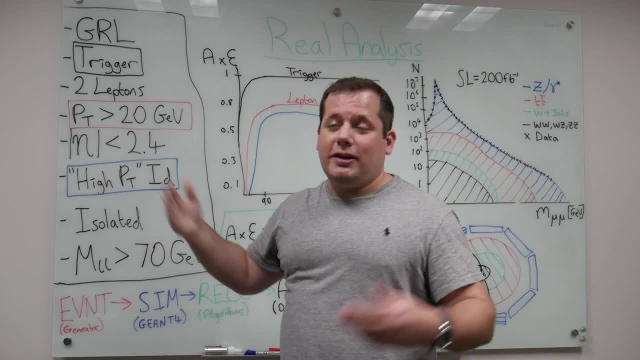 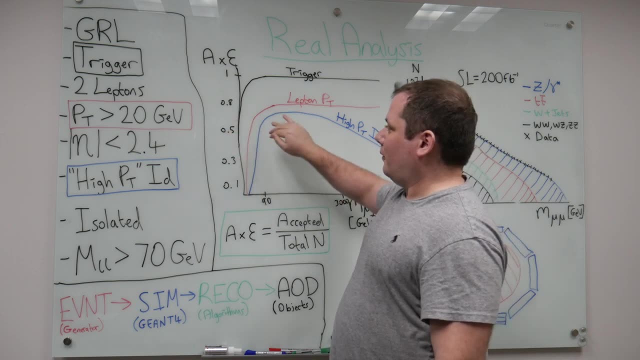 but are higher PT. so here I could use 20 GeV, you could use 30 GeV and therefore, again you see that you're taking a hit. This is now the total acceptance times efficiency. so it's the effect of the trigger and the 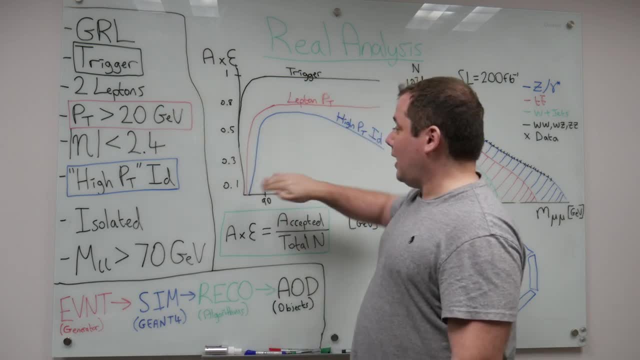 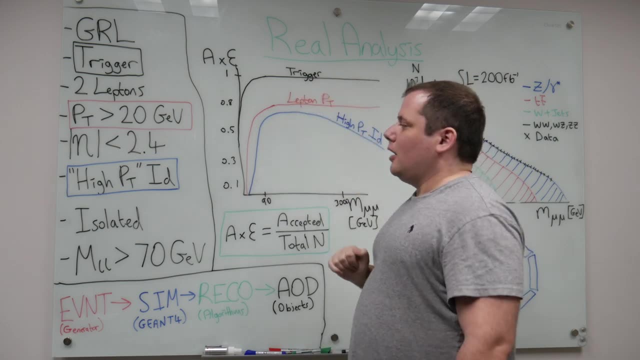 two lepton requirement and now the PT requirement again on top of that. then you can see that our total acceptance times efficiency has then gone down again. OK, Another selection you usually make is to check that the leptons are within a certain ITER. 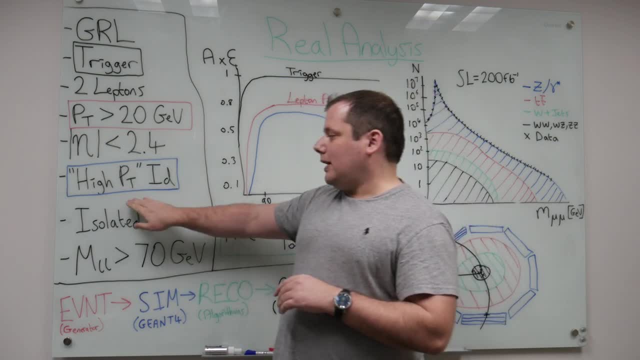 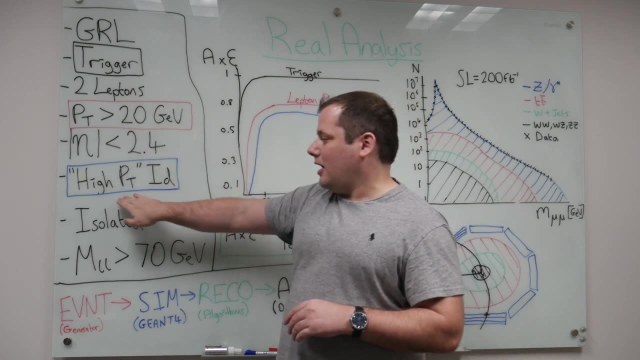 acceptance- we talked about ITER previously- and then one really important concept which is different, apart from the trigger. you know these you've kind of been dealing with before in your truth level analysis, but now you come to some other variables which aren't 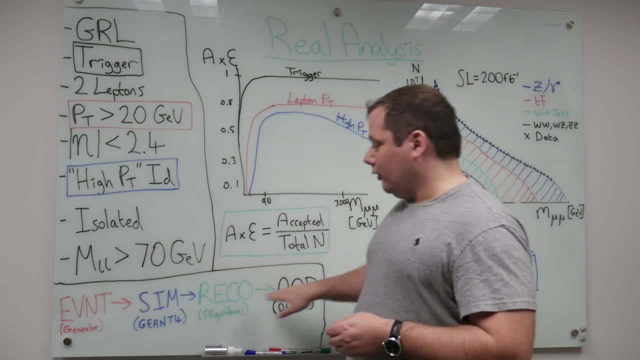 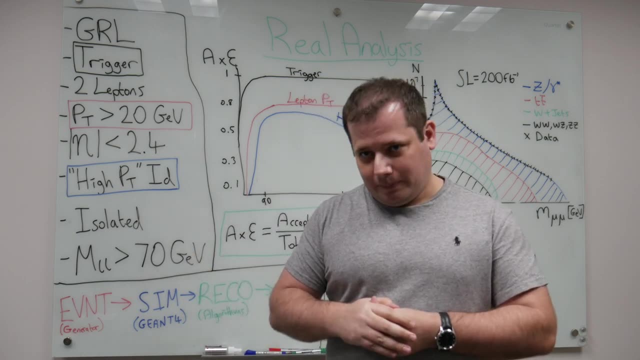 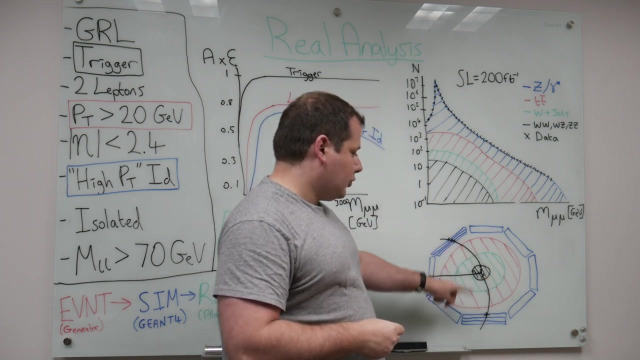 accessible at that truth level. and it's really only when you do this full chain, you get to real life, that you start to see. So there's something here called the high PT identification requirement. OK, The issue is that if we take our detector here and we have muons traversing the detector, 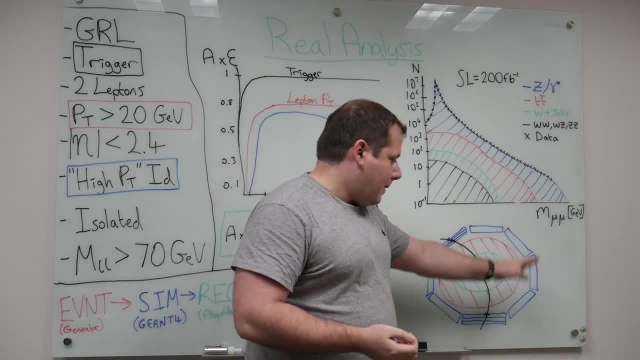 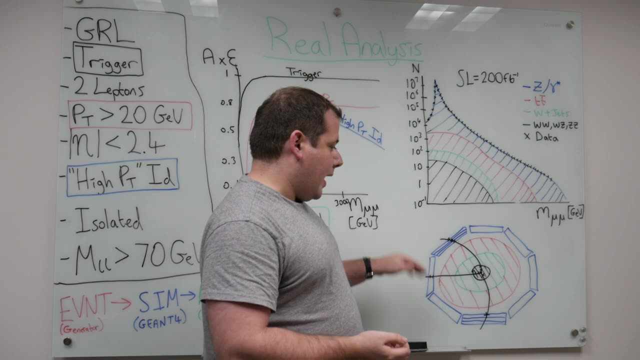 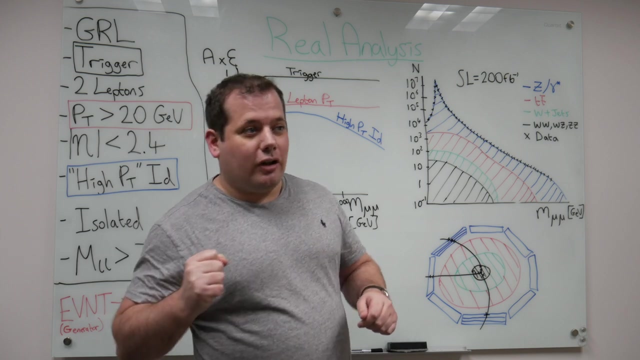 how do we figure out how much energy they have? Well, we're in a magnetic field, and so charged particles will curve in this magnetic field as they traverse the detector and, if you think about it, that the muon has a certain mass, the higher the momentum, the higher the energy, the less chance or the more resistance. 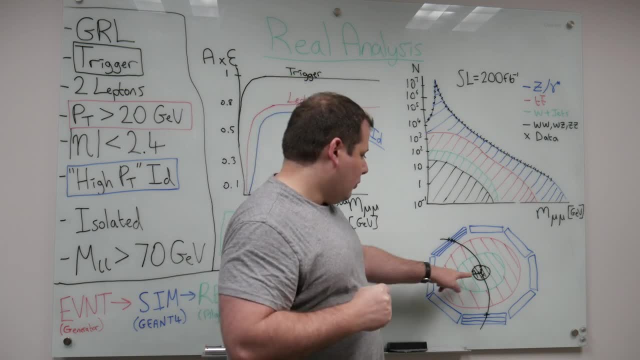 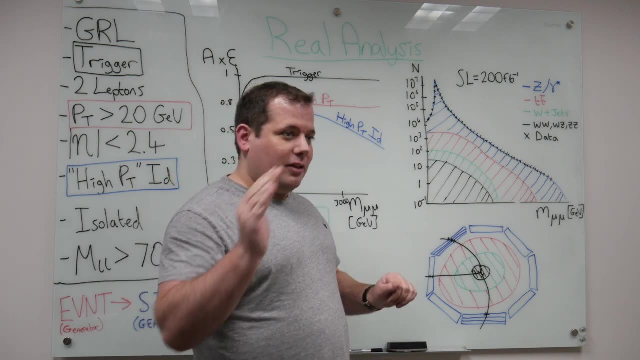 there is to the magnetic field. bending that muon, The straighter muons will be higher energy, right? So lower energy ones. you know, if they're very low energy, the magnetic field can even, you know, make them spiral. 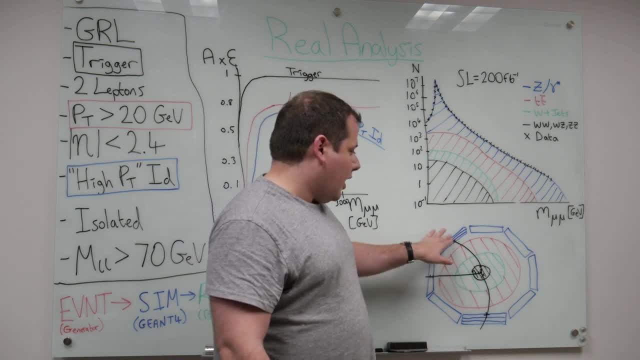 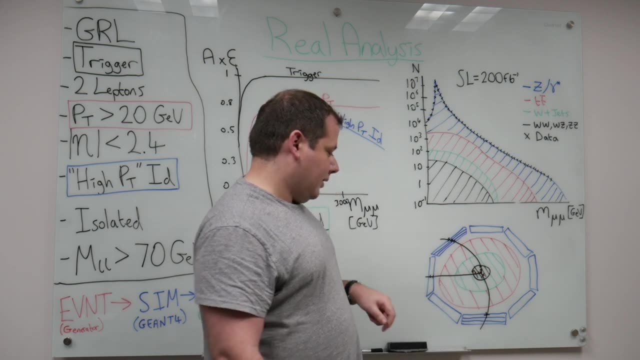 We see that in some cloud chamber experiments, When we get into higher and higher energy, then they leave the detector, but you can see the bending and then the higher and higher momentum they get, the straighter they get. And so one issue is: when they get this straight, you know, how do you tell the difference between? 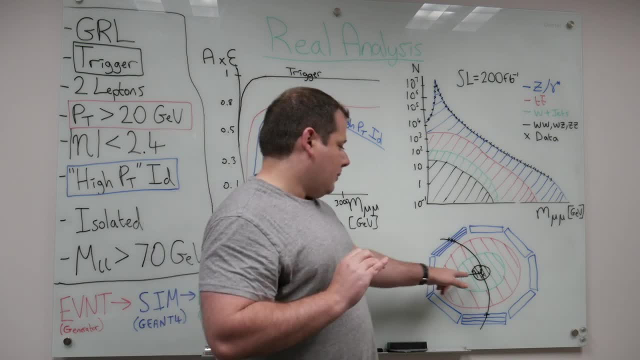 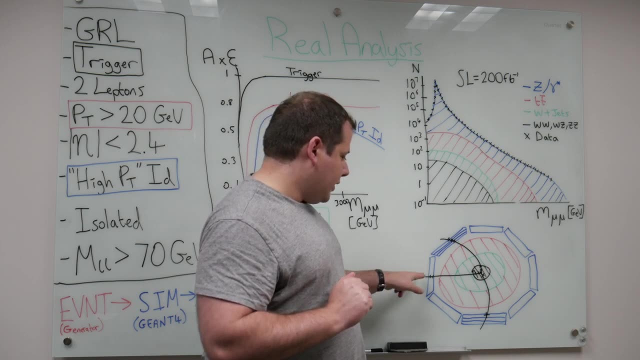 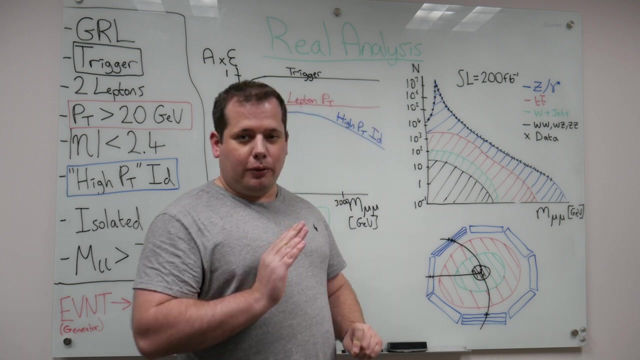 a very straight and an extremely straight track. OK, When we're trying to calculate the energy from this curvature, it becomes extremely hard. And the other thing is, especially when we're- because this becomes so precise, we need to know exactly where that muon traveled through the detector. 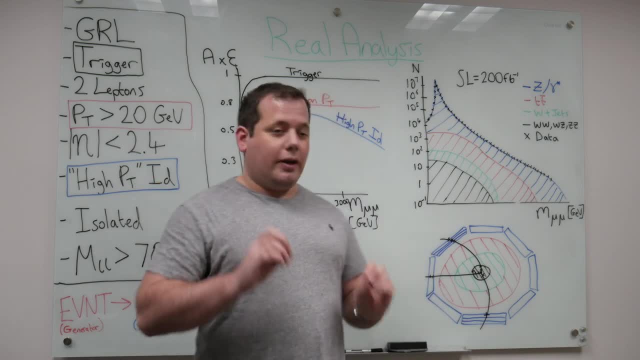 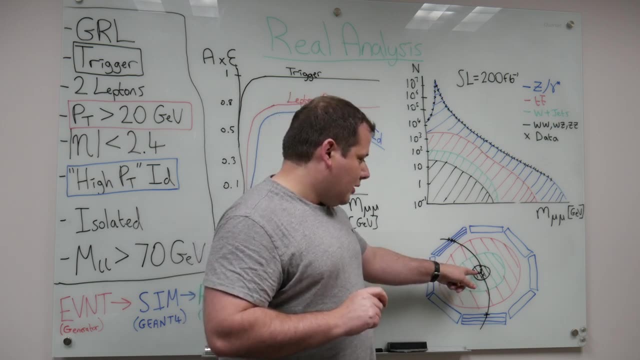 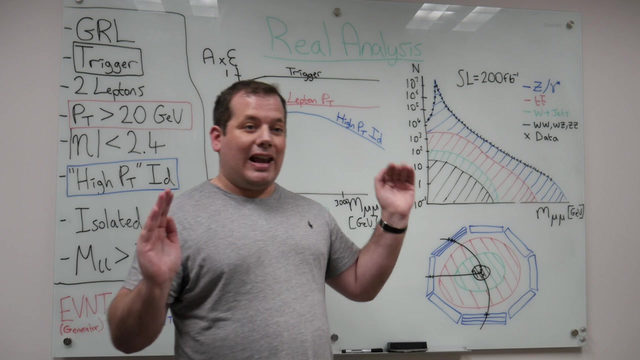 So this high PT muon requirement is requiring that for very straight tracks we have a very good number of hits in the inner detector. So we could say that you have at least five hits in the inner detector and at least three hits in the outer detector, because that allows you to draw a very precise line through. 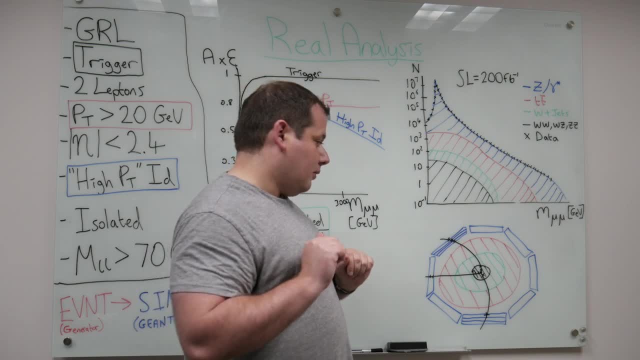 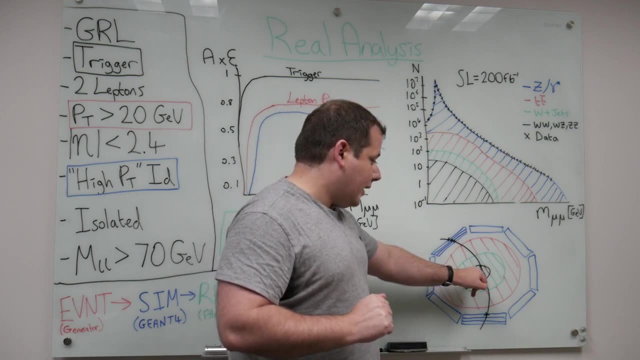 all of those points, You can know exactly where the muon is right And therefore we have a very good estimate of how much energy it has. If, for example, you instead have a muon that only has one hit in the inner detector and 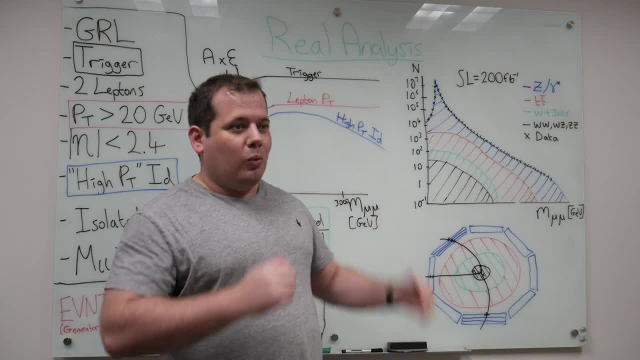 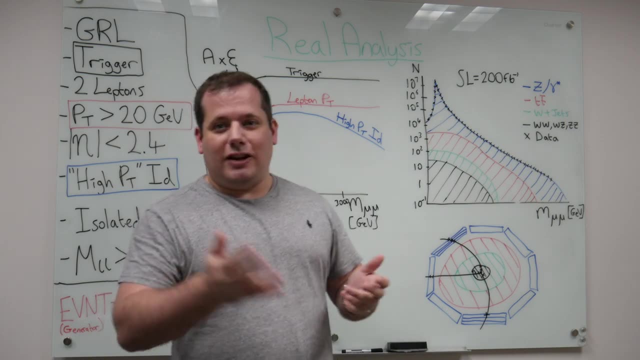 one hit in one of the chambers in the muon spectrometer. well then, the line that you can draw between those points can be very, you know is very uncertain. so the uncertainty on your muon might be very, very high. It might be, you know, hundreds of GeV, even you know a TeV or more. 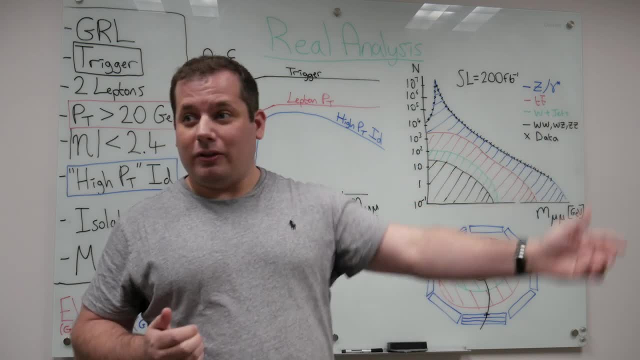 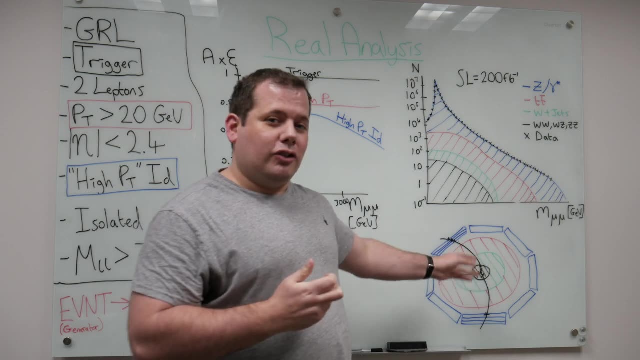 So you could be erroneously seeing extremely high PT muons like 10 TeV, something way off this plot. But it's not because there's really a muon of that energy. it's because the reconstruction has to some extent failed. 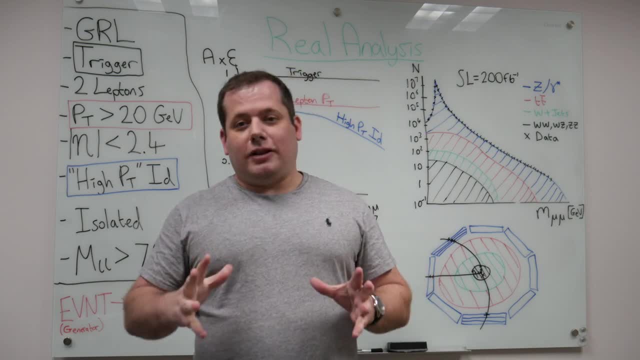 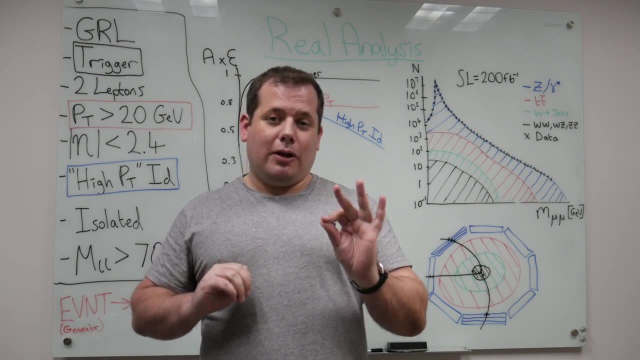 So this high PT muon requirement loses a lot of efficiency. You throw away many of events, but you do that to make sure that the events that you do select are very pure, very low in surface, And this is where you get the efficiency curve. 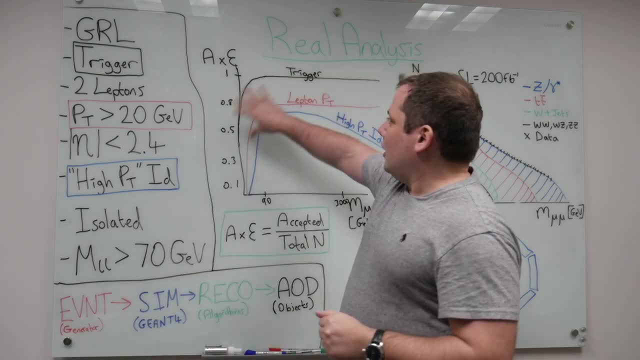 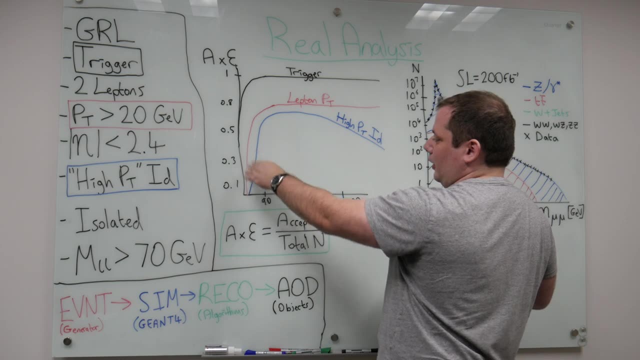 So if you set the efficiency curve you have some quick turn on of the efficiency. there's some losses, right Even for low energy muons. But then you can see, as we get to higher and higher PT, this efficiency starts to drop. 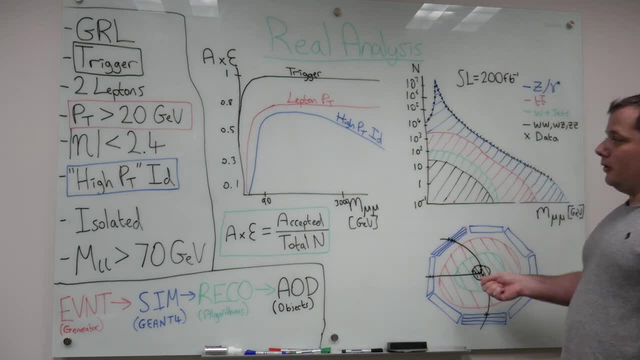 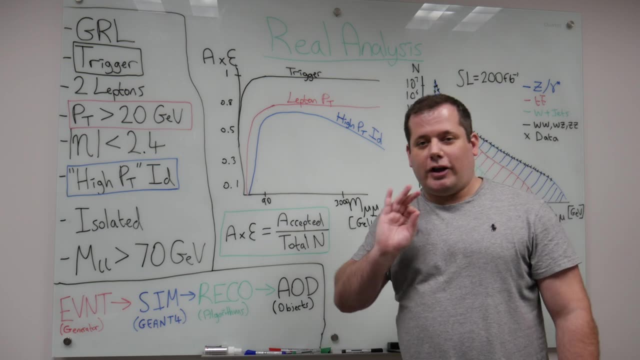 off because it becomes harder and harder to identify these muons right at higher and higher PT. However, even though we're throwing many away, we're keeping the ones which are like the golden channel, The ones that we can really trust. 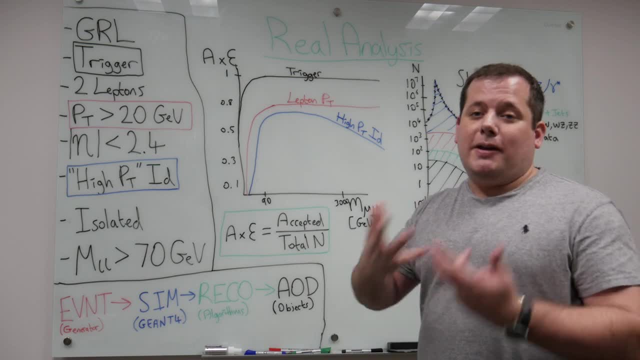 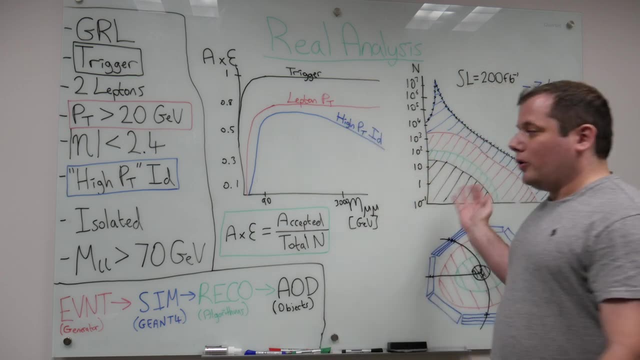 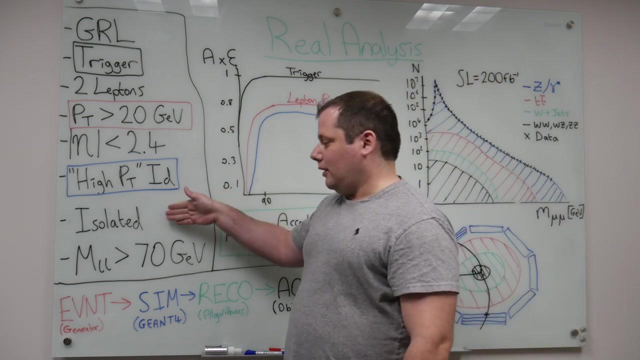 and that can sometimes be more important than just keeping as many muons as possible. This is something that's continually being worked on: trying to improve this while not sacrificing. you know the robustness of our estimates, And there are some other concepts here. One is: you can just make an invariant mass. 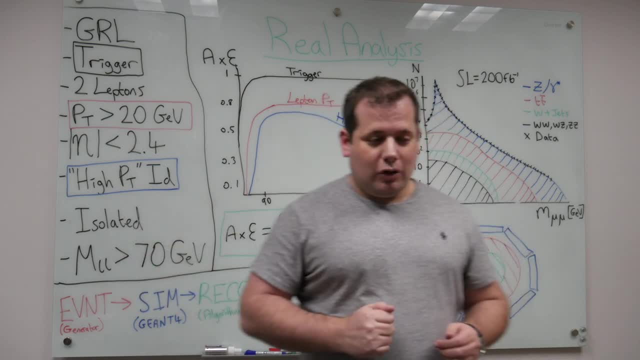 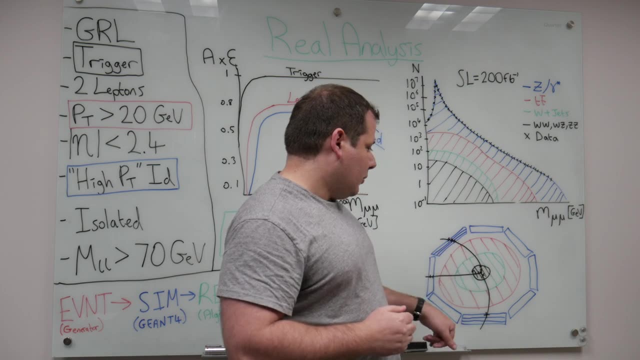 cut and the other one is about isolation. This is more relevant to electrons, but you can look in the detector at how much energy is around your object as it passes through, because maybe that muon is inside of a jet right and maybe that's. 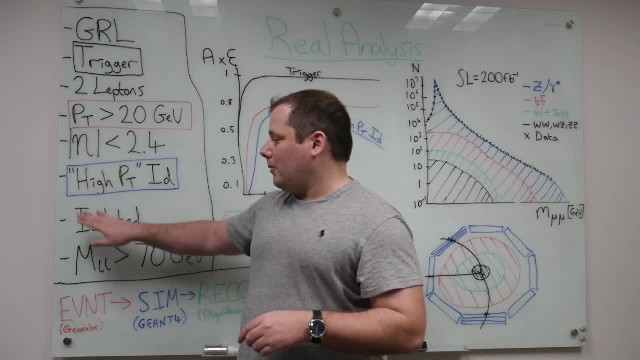 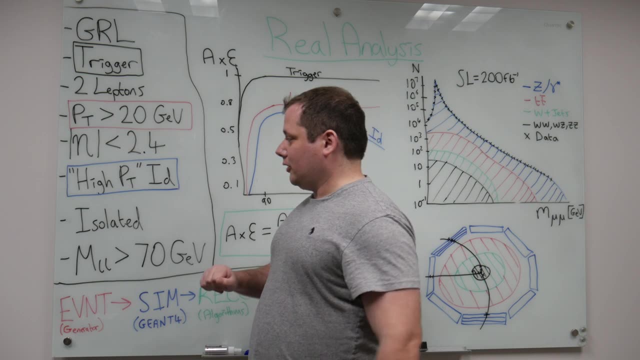 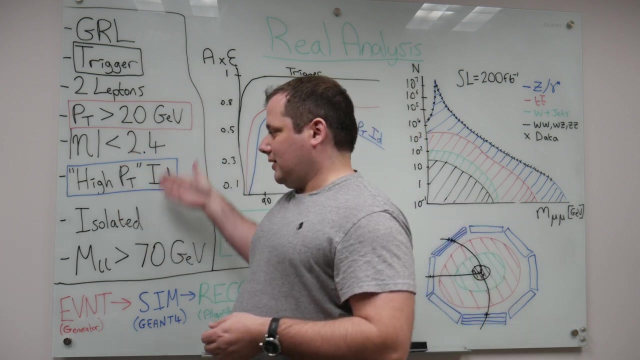 throwing off your calculation. So generally, we ask that there's not much energy deposited in the detector around our objects. so again, we know that we're making a precise measurement. it's not adding extra noise. So this is when we go on to perform a real analysis. this is more what the event selection will look. 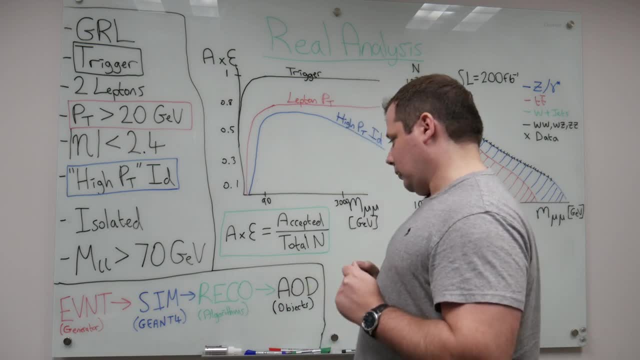 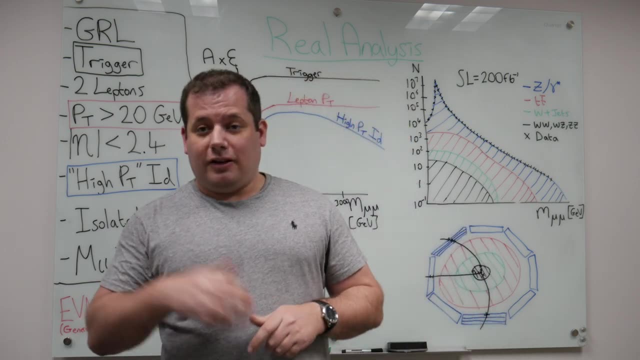 like, and we're going to look at what the event selection will look like and we'll get us as close to the data as possible. okay, And so when we go on to this next stage, you will actually be performing this on many physics processes and 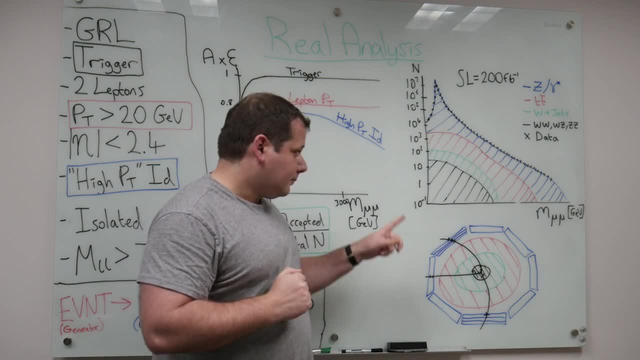 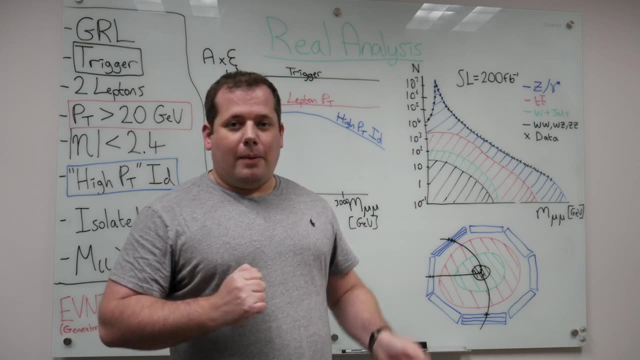 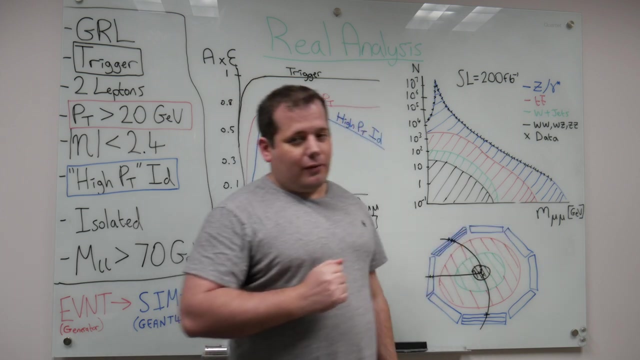 running over the data so that we can make a comparison between them Now, up till now as well. you've only been looking at the z-prime signal and I mentioned in the previous talk about the standard model distribution that you would see. So let's go back to our friend here, the di-lepton invariant mass. 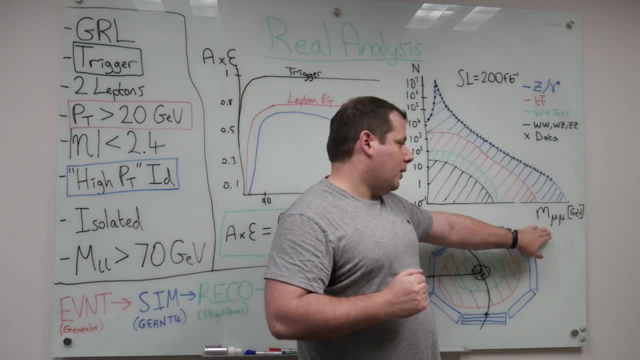 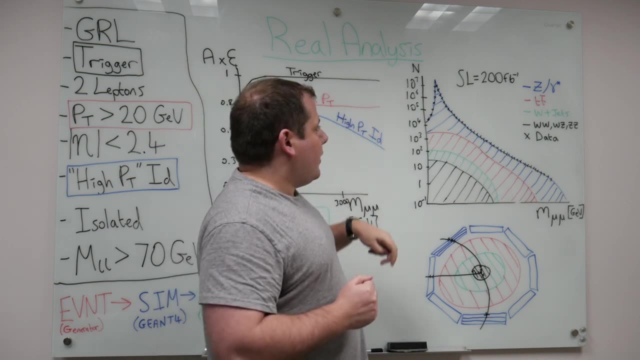 distribution. and again here we're going to be looking at the z-prime signal. and again here, this time I'm talking about two muons, okay, and now I've even drawn a scale on the y-axis, so the number of events here I've gone up to ten, to the 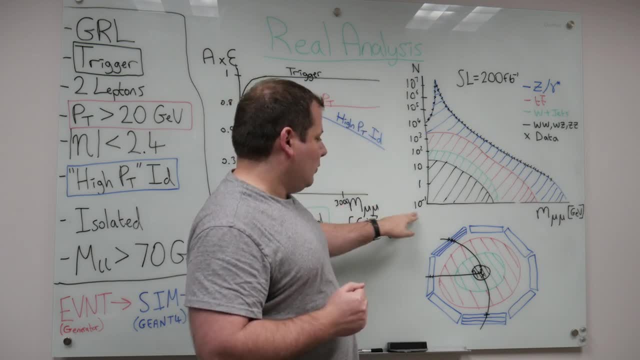 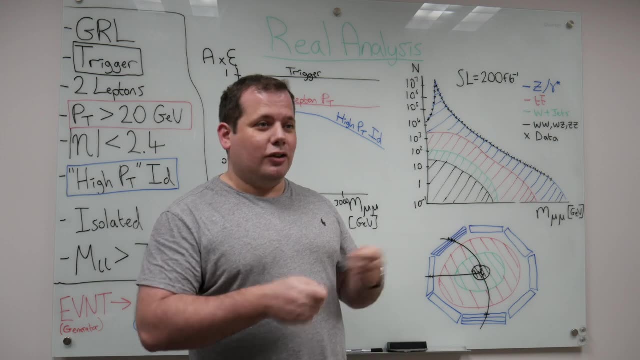 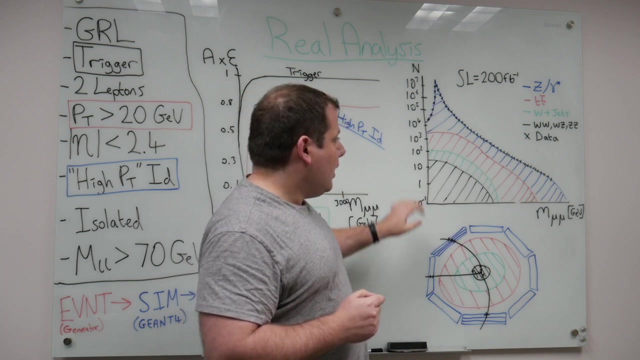 seven events, and you can even scale it to less than one. you can have ten to the minus one events here. you just would never expect data to be fractional, because of course you only see integer numbers of data events, but you could still scale your Monte Carlo to any number you like. And now, instead of just 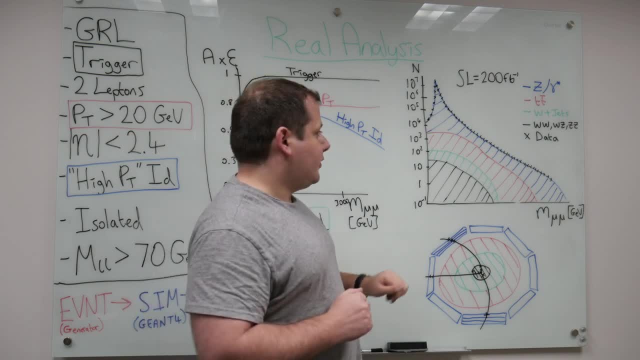 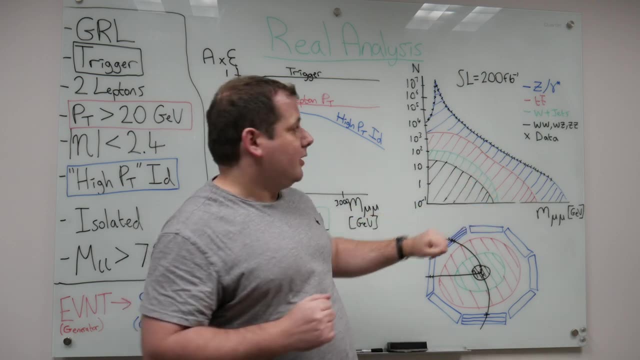 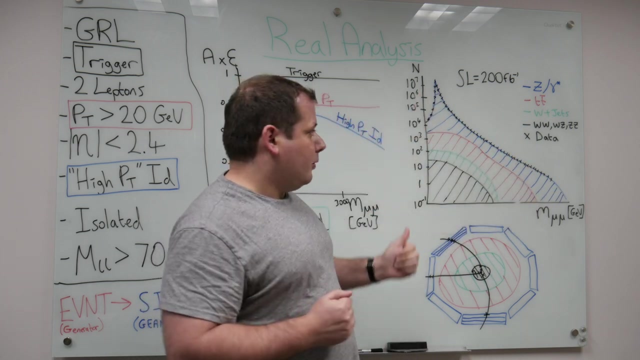 having that one black line showing you the falling distribution. what I've actually split it apart into now is all of the different standard model processes that you would see when you're looking in this channel. So still by far the most dominant process that you would see in proton-proton collisions at the 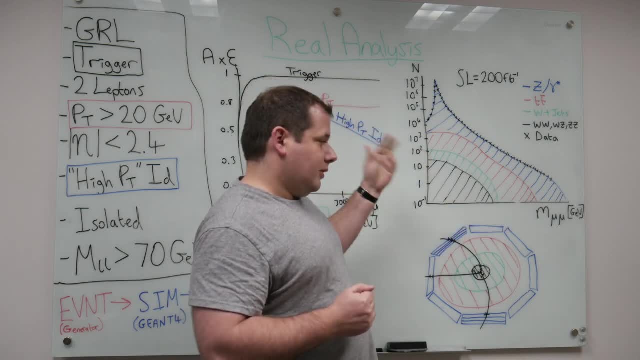 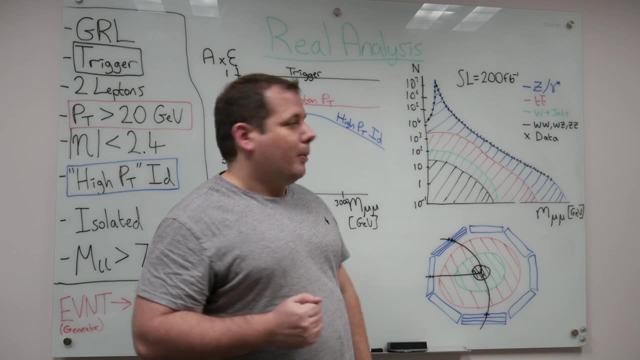 LHC. looking in this channel for di-muons, the same as for di-electrons, you would see the z and gamma process. so you would see standard model z bosons being created, decaying to two electrons. However, you would also see other 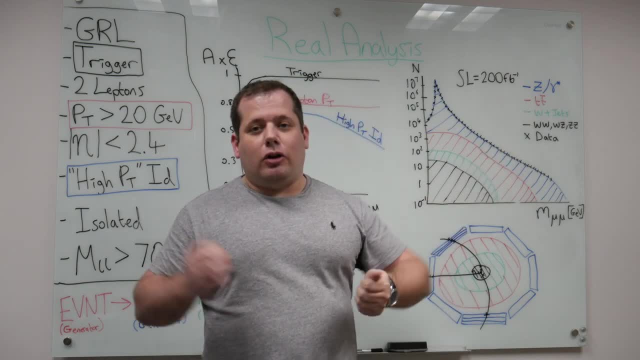 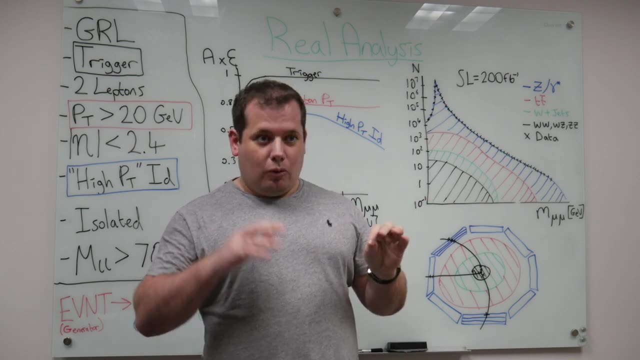 processes as well. so you would have TT bar. so I'll let you look up more about that process. but essentially the each top quark can decay most of the time, almost entirely of the time, to a W boson and a B quark and that W boson then 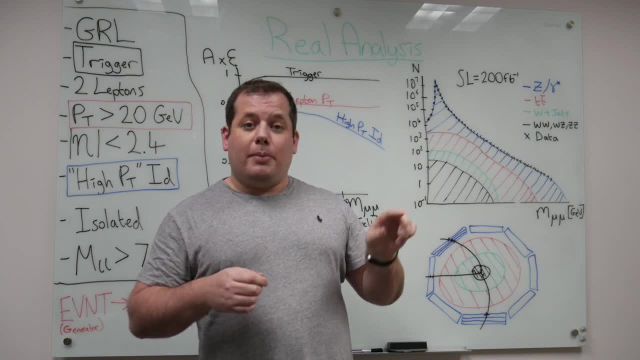 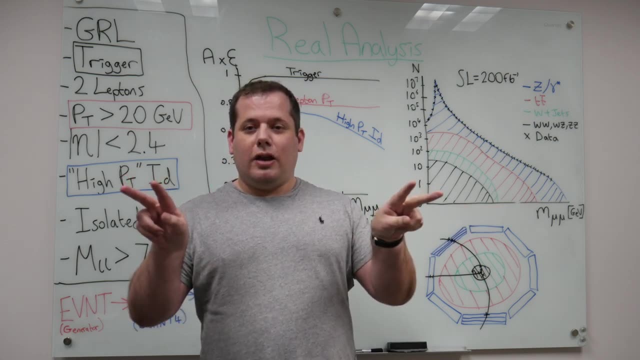 can further decay into other things, such as quarks, but including a lepton and a neutrino. So if you had two top quarks that both decayed to two electrons and then both of those Ws decayed to a lepton and a neutrino, well, you'd have two. 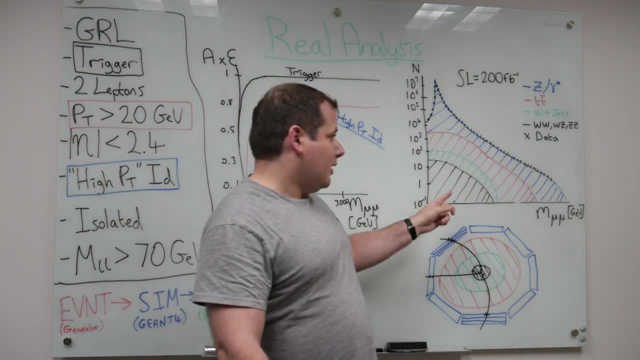 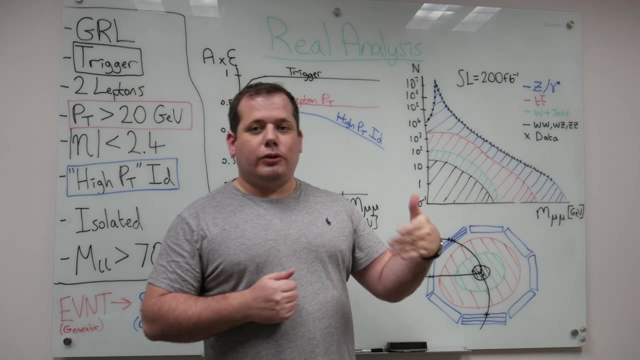 leptons in the event, so you might pick up some of those events in your selection. Now, because of things like the isolation requirement, you hope to minimize those number of events, but some will still sneak through into your selection. So, as well as running over a standard model z simulated sample, you 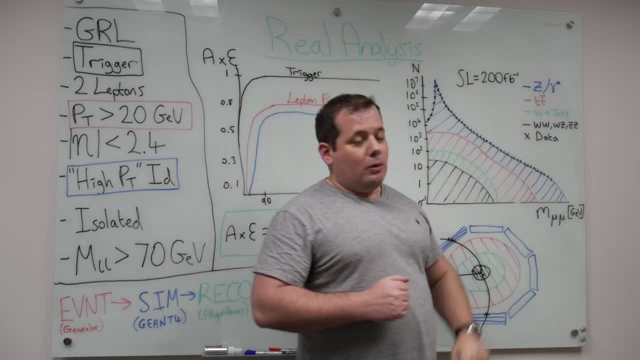 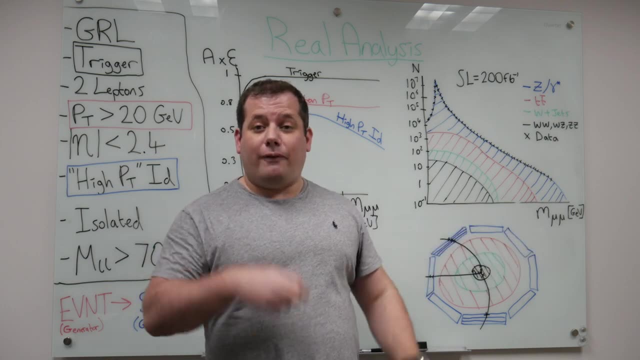 need to run over a TT bar sample. you could have W plus jets, so where a W boson that decays to leptons is produced in association with jets and one of those jets might fake an electron or a muon. much harder for muons, but very 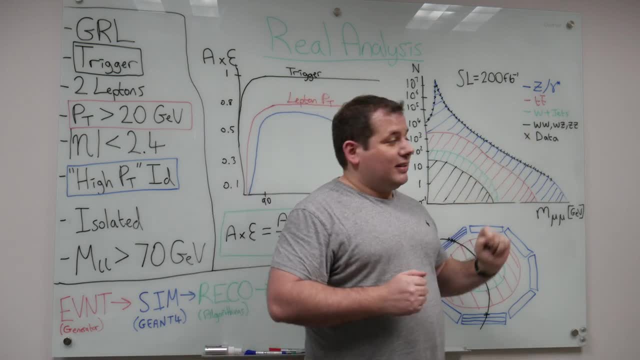 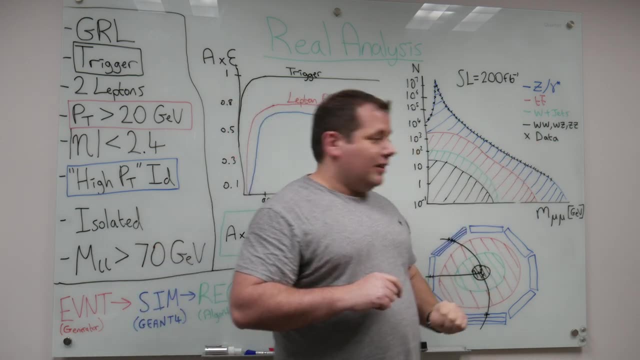 common for electrons. and then you can even have other processes, like diboson process, where two Ws are created which both decay to leptons, or maybe a W and a Z is created, and you know, there you could potentially have the Z decaying. 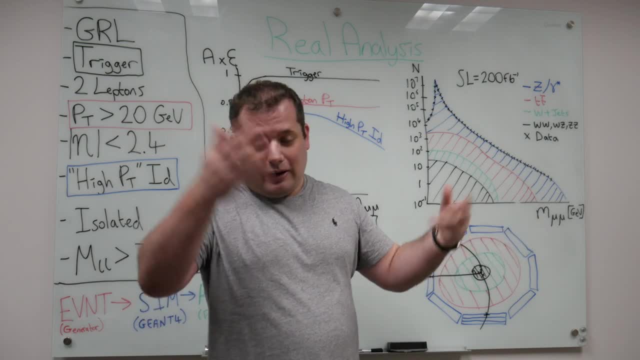 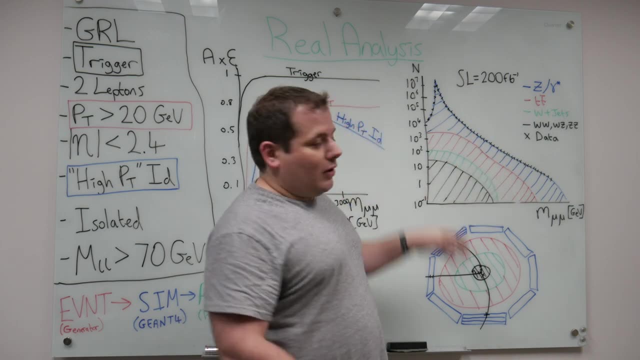 to leptons and the W decaying to quarks or leptons, so you could have two or even more leptons in the event. So all of these have been stacked on top of each other to give us the total estimate from the standard model, what we would see, and the reason we do this is because 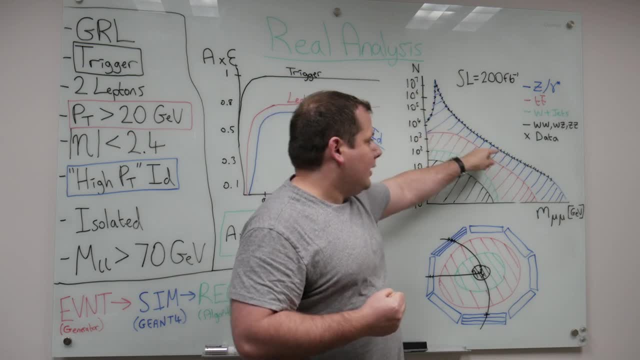 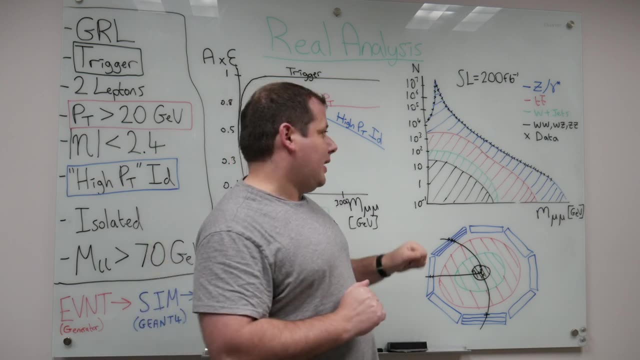 then when we run the real data here which is in the black little crosses here, so you can see I've drawn my legend, just like you recently did when you made your nice plots with the truth level analysis, with the black points here for data, we 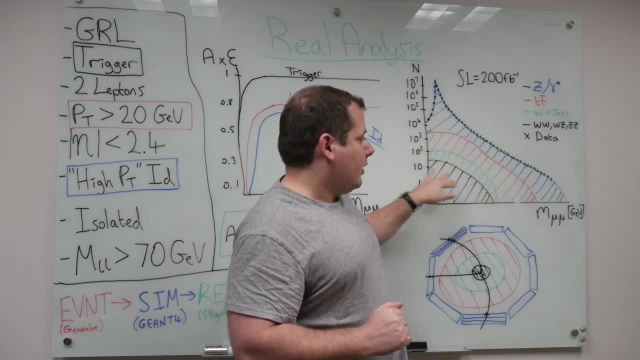 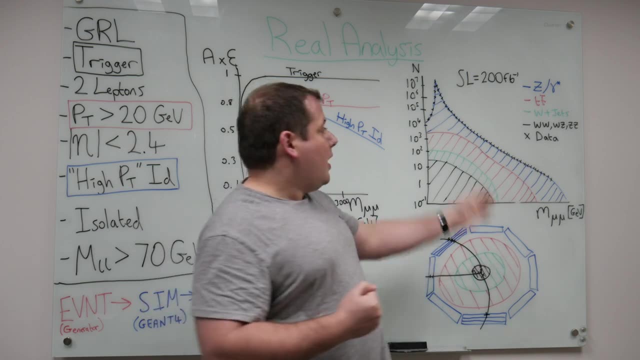 want to get as close to the full simulation as possible, right? This is. all of these colored diagrams represents our best knowledge of the standard model and we're comparing it to the data and we want to try and understand as precisely as possible. if 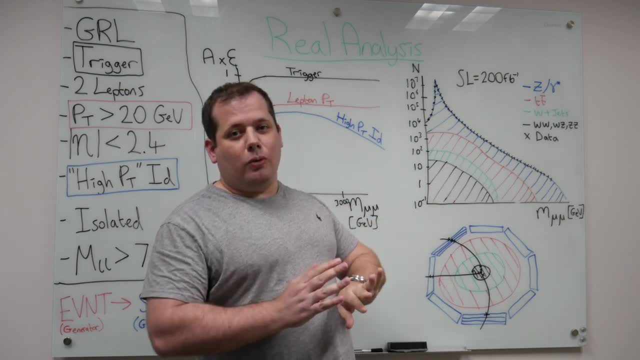 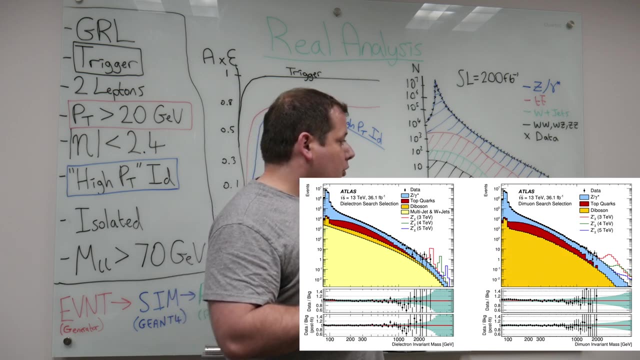 that matches Now at this point- probably down in the corner, I will flash up a real image of this, not just one that I've drawn, but one from a real analysis that was recently done and you can see, usually there there's a ratio subplot which shows 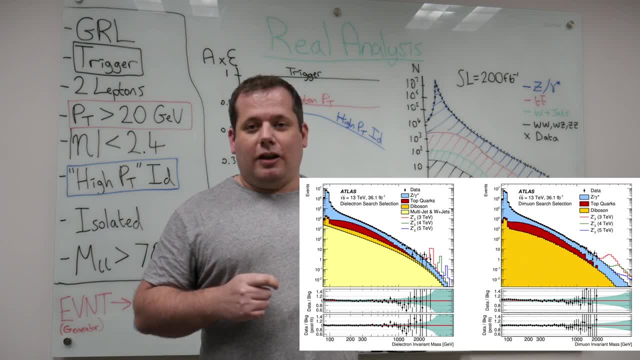 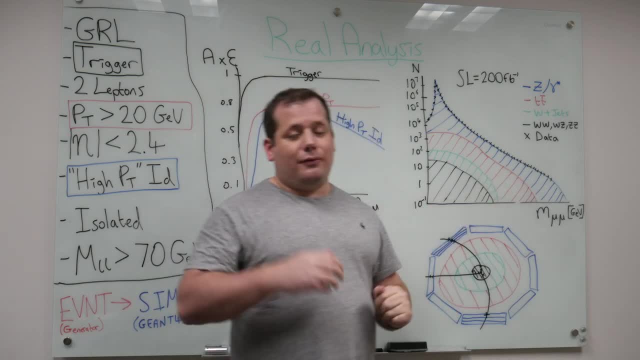 you the ratio of your estimate- simulated estimate- compared to data and you can see that generally the agreement is good, which means up until now we haven't found any new physics out of high mass, but with the more data we collect, we're populating these. 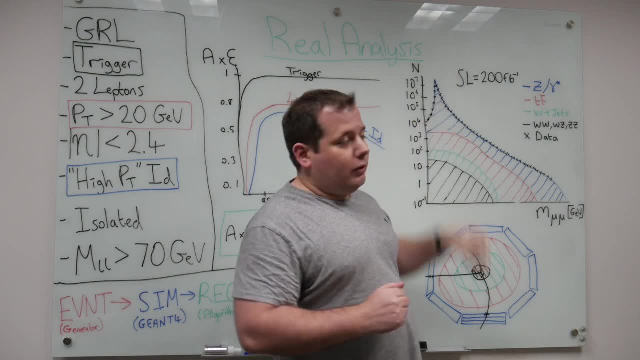 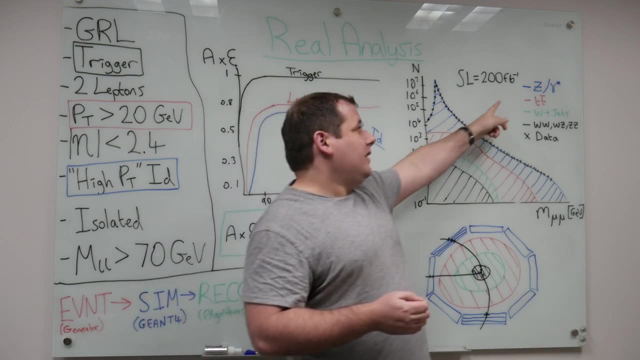 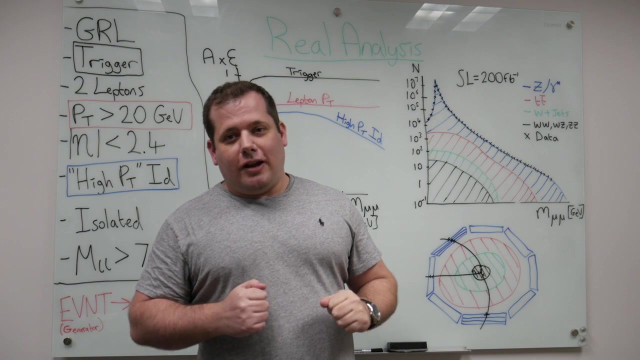 tails. so I've drawn here an integrand symbol with L for integrated luminosity, which has units of inverse barns. here for the scale, we've gone to inverse Fenter barns and so currently, at the LHC of Time of Writing, we've collected around 139 inverse Fenter. 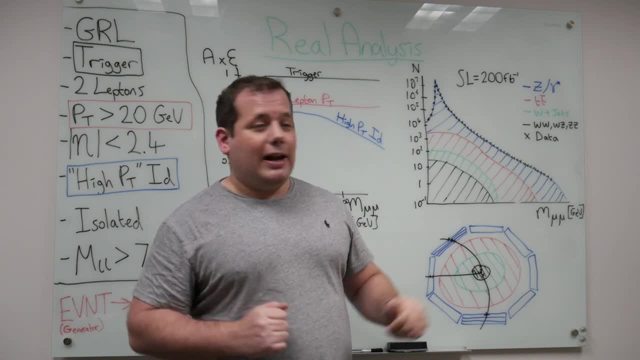 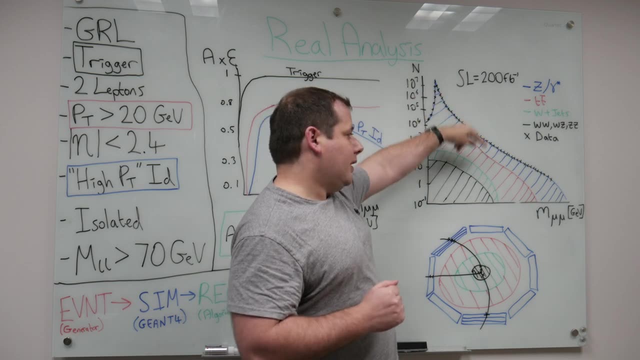 barns of data, and now we've just started run three, so we're collecting even more data. but essentially, the more data you collect, just think of it as the more events that you're putting into these bins, right, so this whole distribution is going to be moving up in. 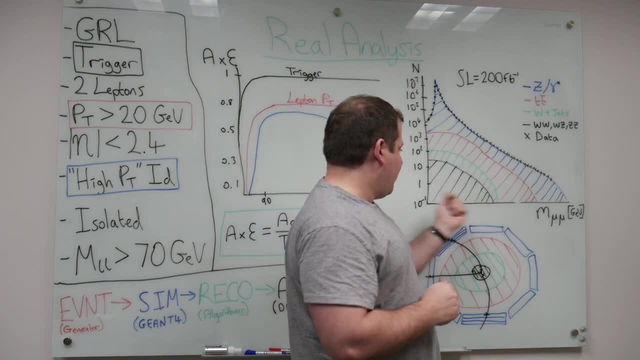 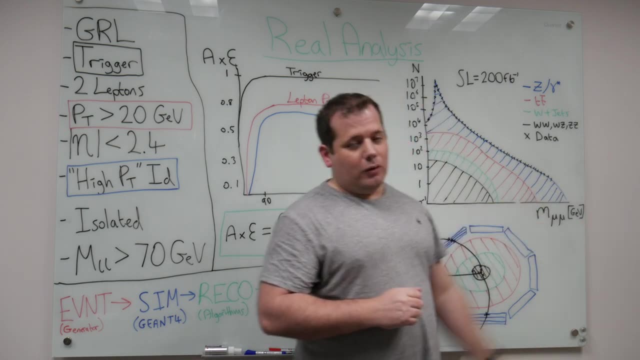 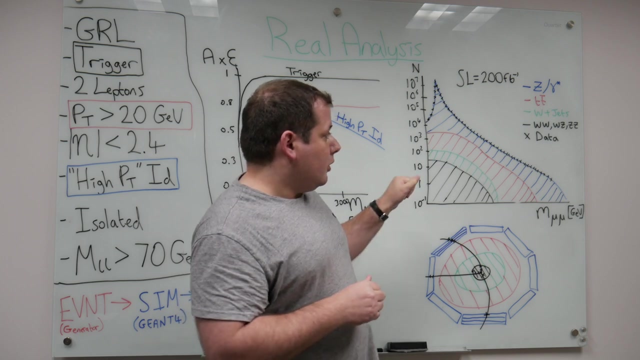 the number and you can imagine as this number moves up, then you're expecting around one event out at high mass, and the higher up it goes, the more you expect events to be filled out in this tail which allows us to search for new physics at higher and higher mass. So you know, this is the. 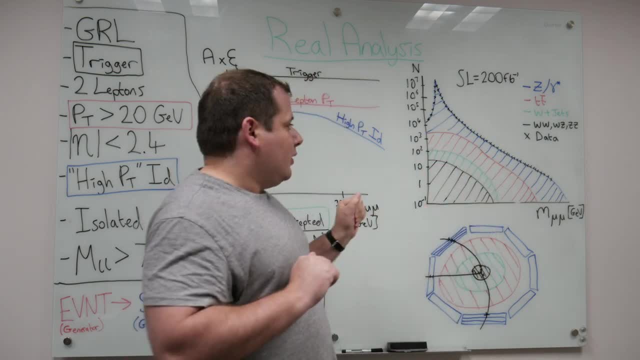 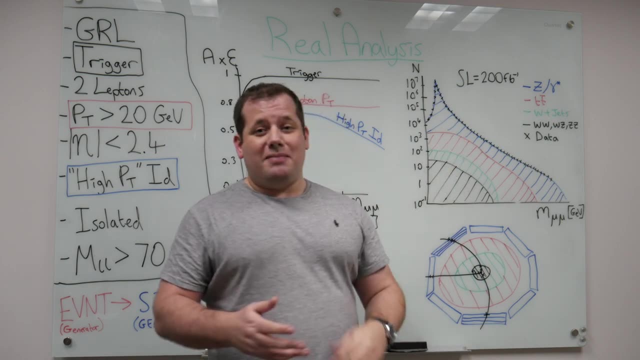 big picture of what we're heading to next, but in reality, you know, I'm not going to ask you to go through this whole generation chain for all of these different processes, and you will also need millions and millions of events to be able to, you know, have an accurate simulation. you know, here we have. 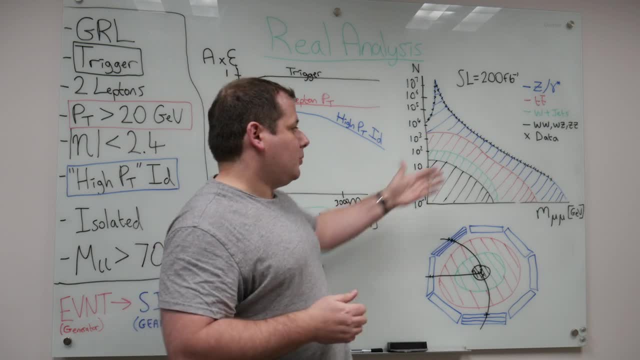 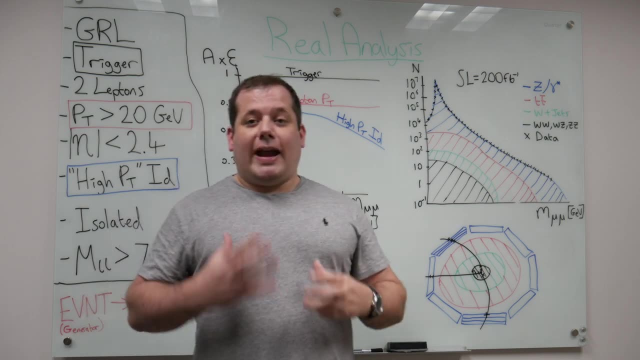 roughly ten to the seven events, right, so you can imagine how many events we have to generate at Monte Carlo to be able to appreciate that. okay, So in reality, there's also a way that you can download samples that people have already generated. in fact, there are whole groups of you know, tens to hundreds of